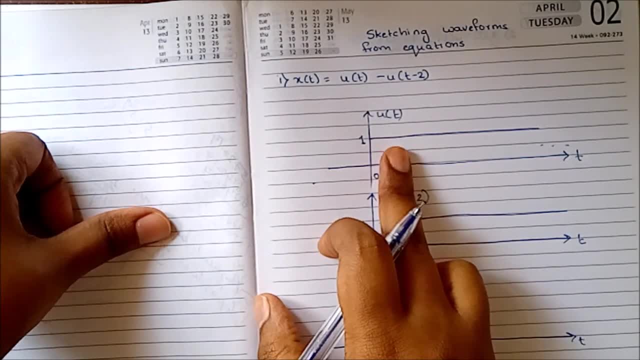 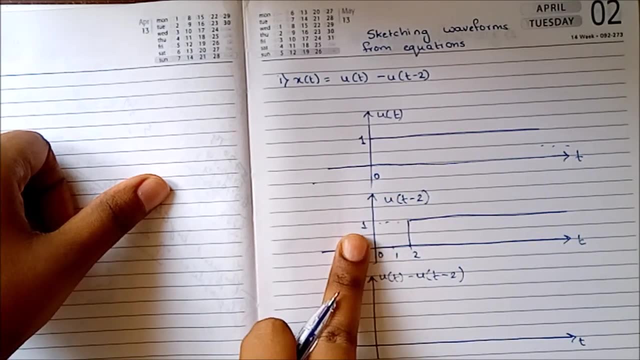 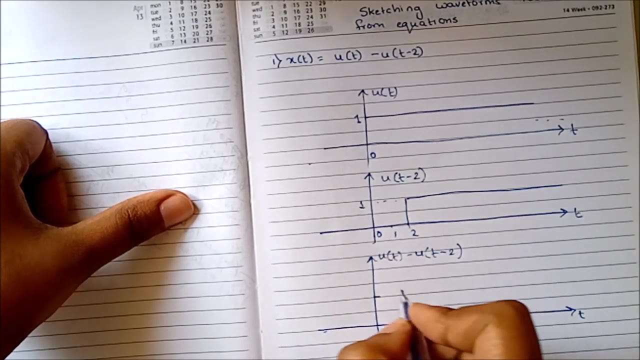 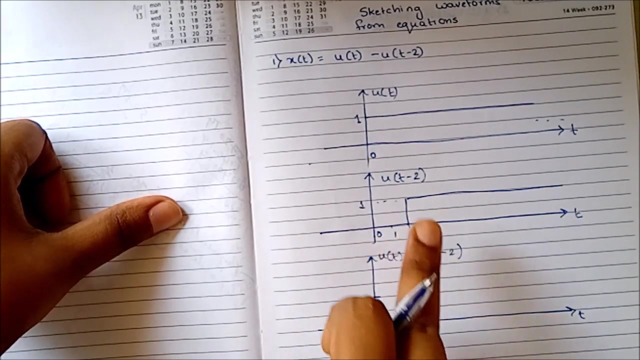 Both are zeros. At 0, the first signal has an amplitude of 1 and the second signal has an amplitude of 0. So 1 minus 0 will give us 1.. So the resultant signal will begin at 1.. At 1, the first signal again has amplitude 1 and the second signal has amplitude 0. So 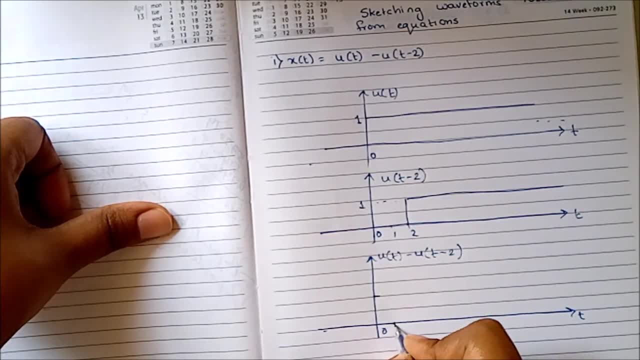 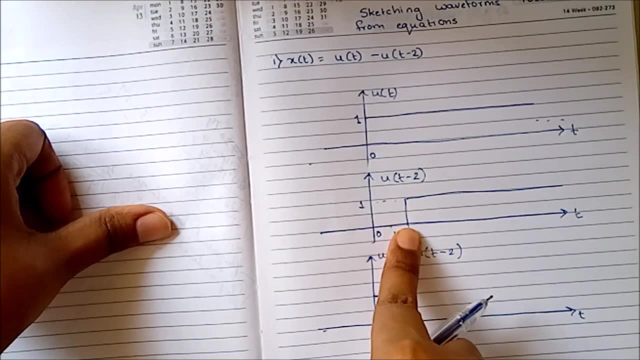 1 minus 0 will be again 1.. At 2 the first signal has amplitude 1 and the second signal also has amplitude 1.. So it will be 1 minus 1, so 0.. So this is 1.. So this is 1.. 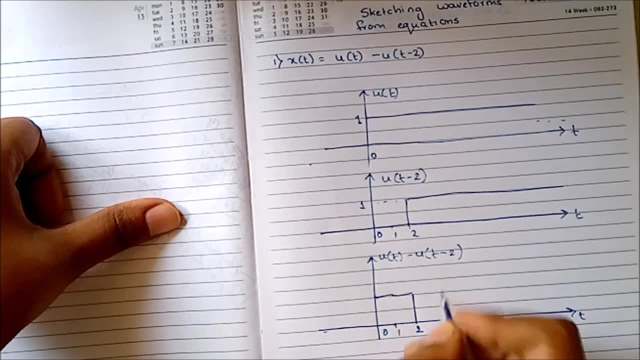 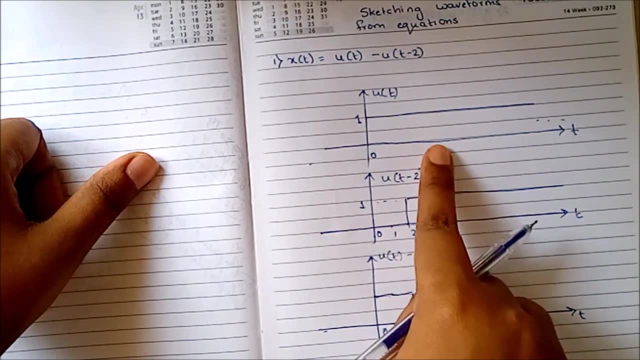 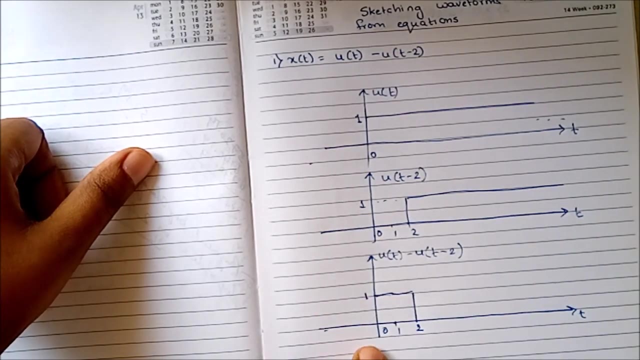 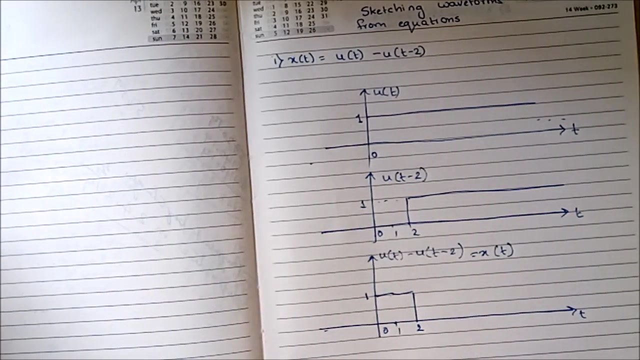 At 3,, 4 and all the other consecutive values. we have the amplitude as 1 for both the signals, So the resultant signal will be 0 at all the other points. So this is the result which we require. So this is x of t. 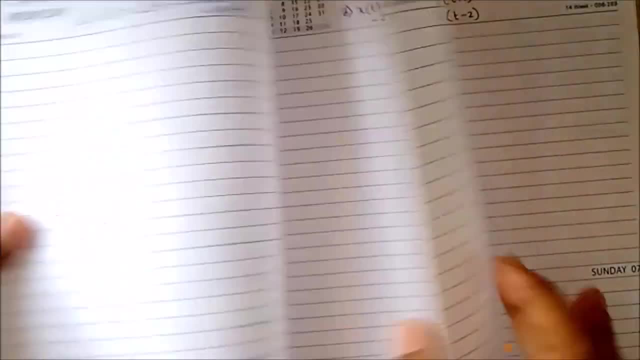 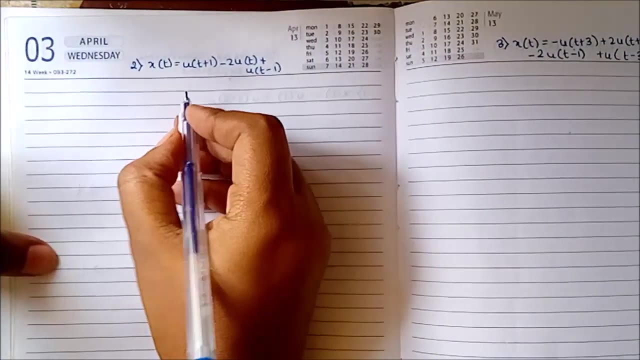 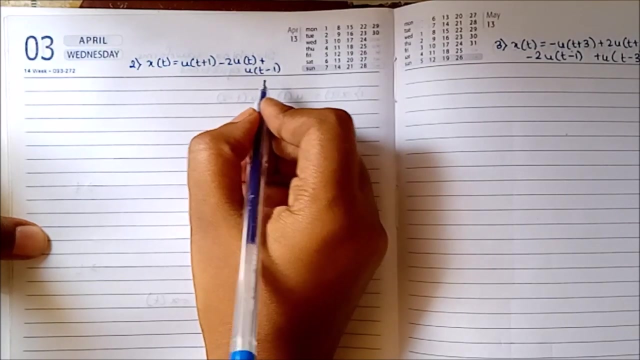 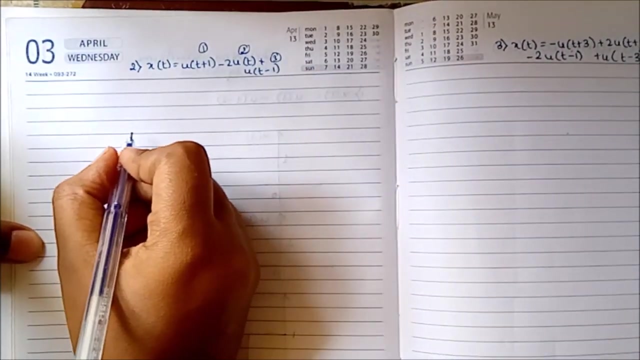 Now we will solve the next. x of t is equal to u of t plus 1 minus 2, u of t plus u of t minus 1.. So this is the first signal, second and third. First let's draw u of t plus 1.. 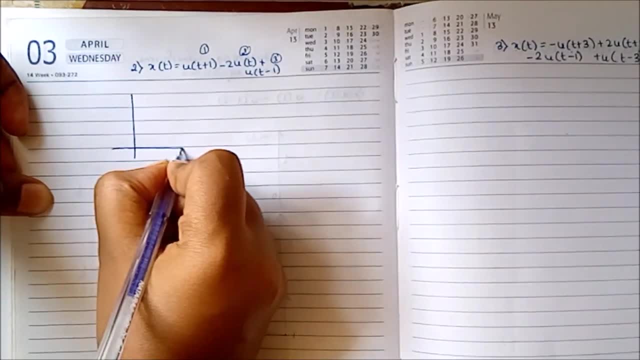 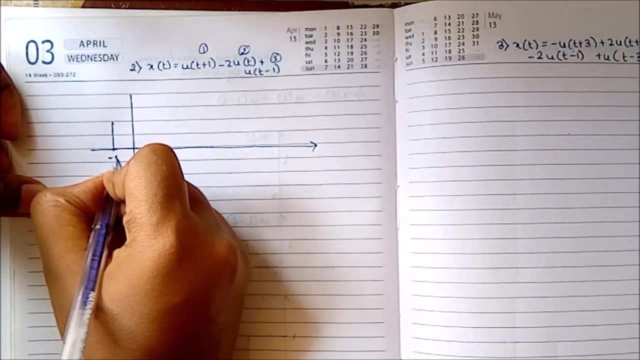 This is an advanced version of the unit step signal by 1.. So this is the first signal, This is the second and third. This is the third, This is the fourth, This is the fifth, This is the sixth, This is the sixth. 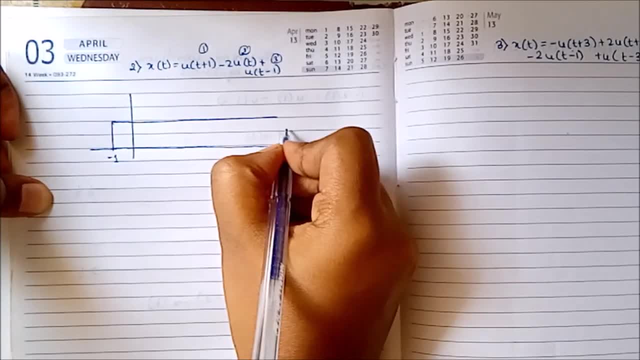 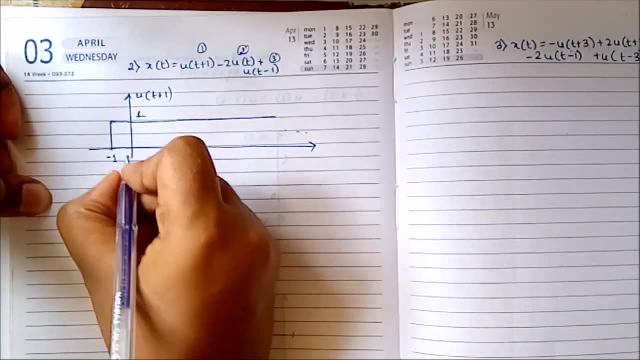 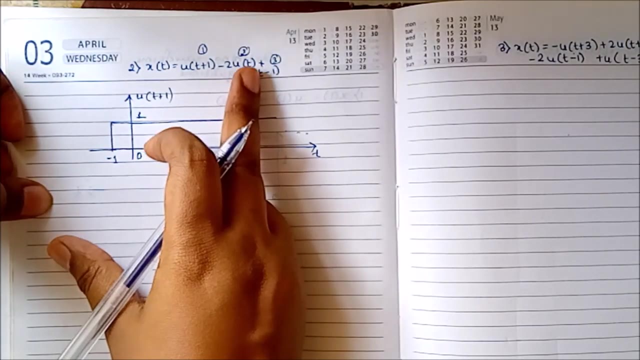 So it will start at minus 1 and will continue to infinity with amplitude 1.. The next signal is 2 u of t. So this is the unit step signal amplitude scaled by 2.. So the amplitude will be 2, but it will be the original unit step signal. 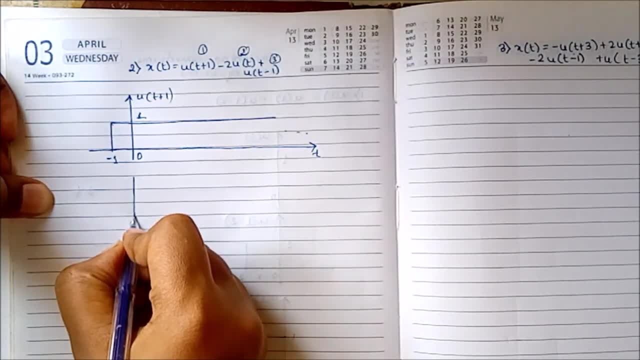 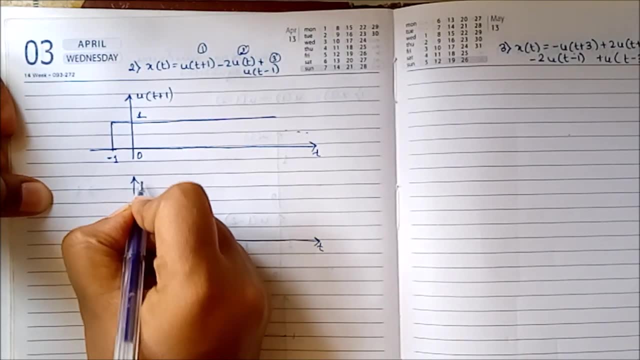 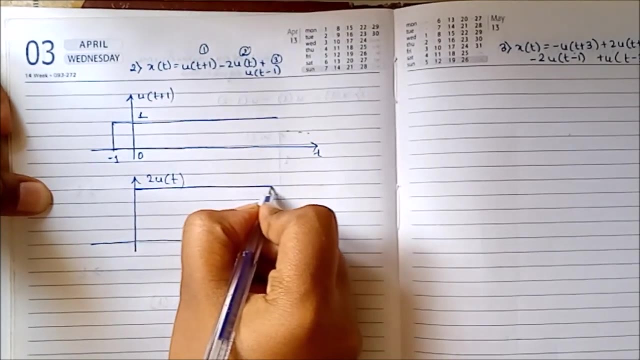 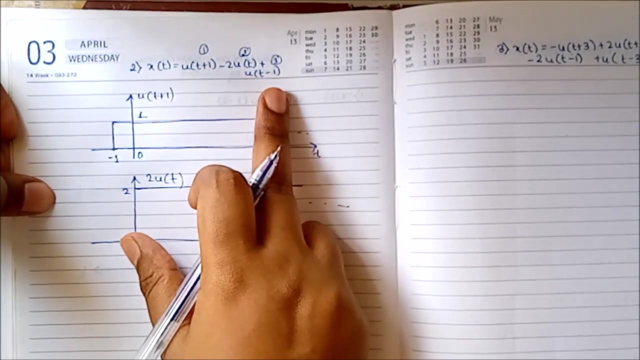 So this is the unit step signal Amplitude scaled by 2.. So this is the unit step signal 2 u of t with amplitude 2.. This will continue, And the third signal is u of t minus 1.. So a delayed version of the unit step signal by 1.. 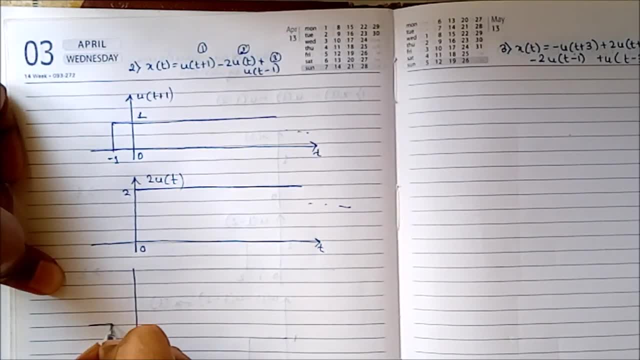 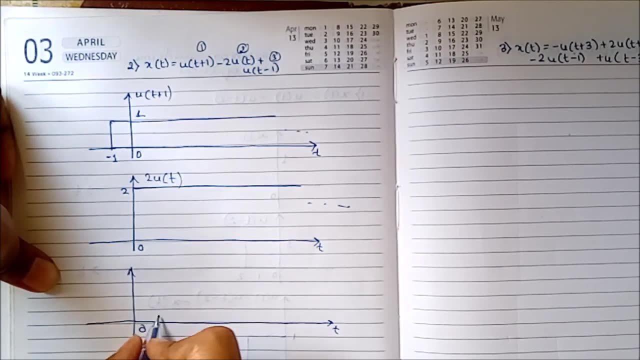 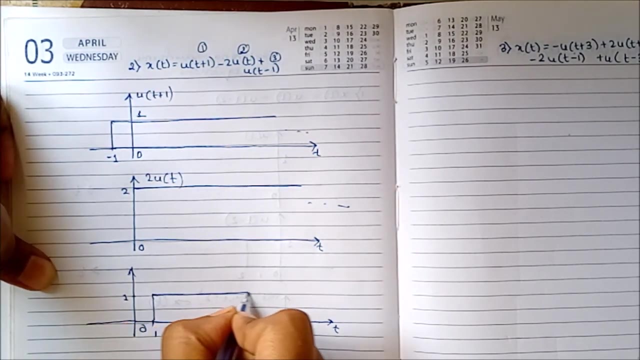 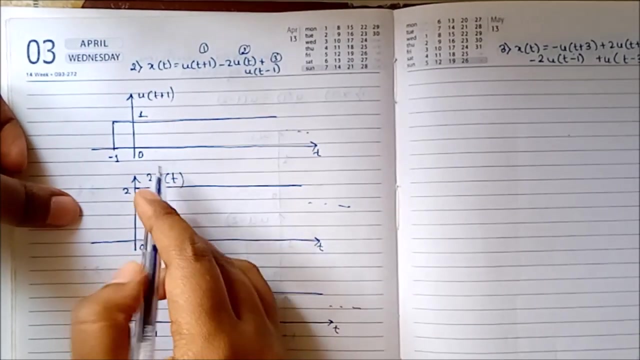 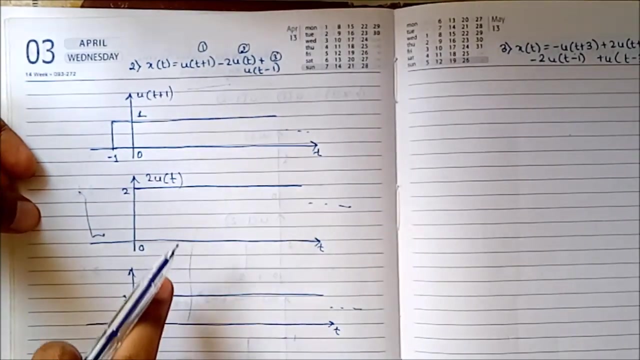 So the amplitude will be 1 and the signal will begin at plus 1.. Now we have to perform the operation. We can either take these two signals first and perform the first part of the operation And then the second, or perform all together. 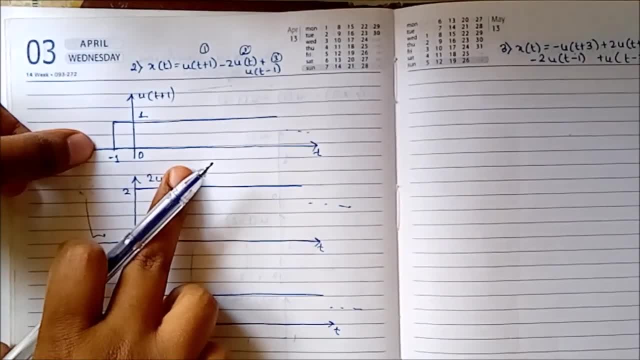 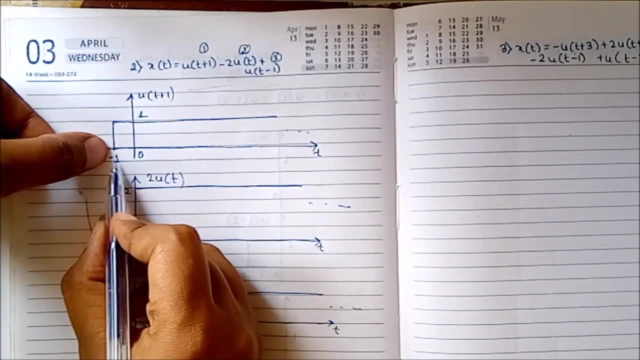 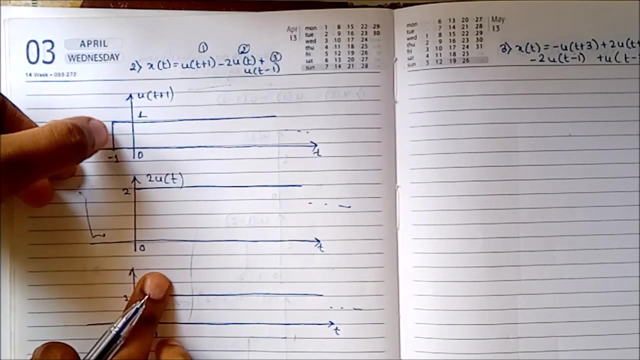 So first we have to subtract the second from the first and then add the third signal to it. So let's do it. So the first signal is starting at minus 1.. The second and third signals: they are starting after that At minus 1. the first signal's amplitude is 1.. 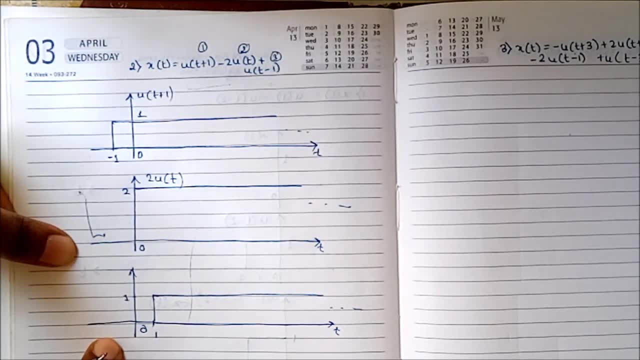 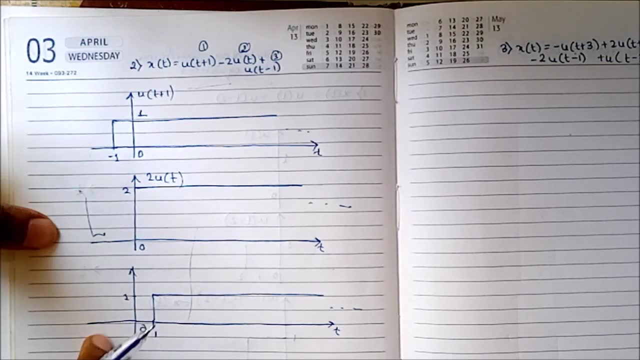 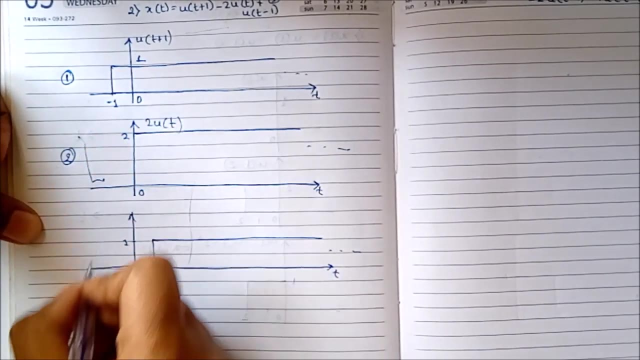 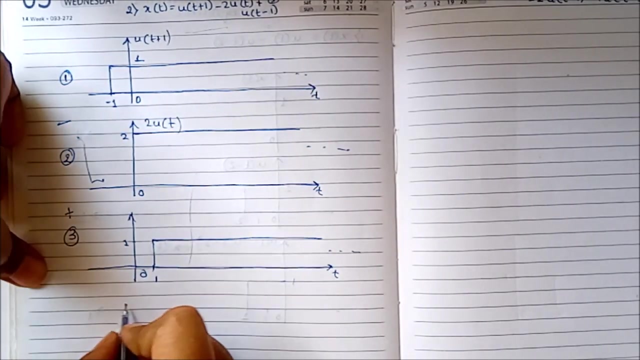 And the second signal's amplitude is 0.. Third signal's amplitude is 0.. So 1. Minus 0 plus 0 is 1.. So the resultant signal- we will just name these So 1 minus 2 plus 3.. 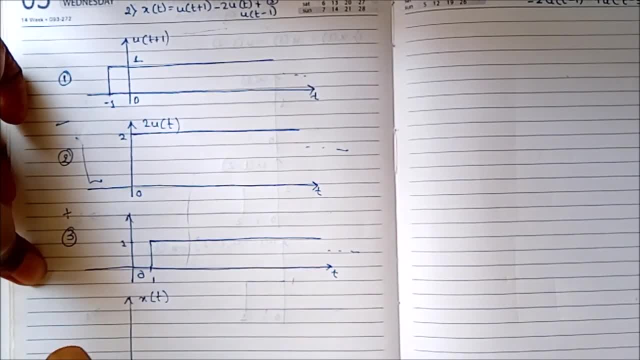 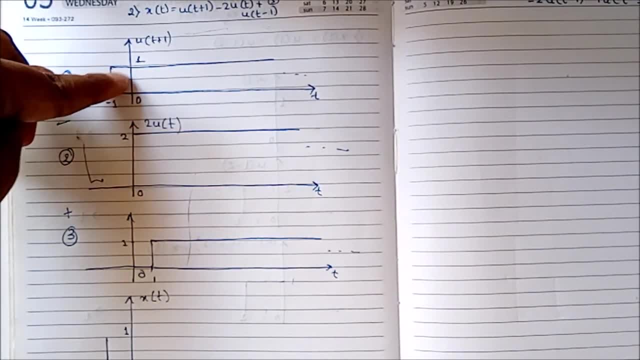 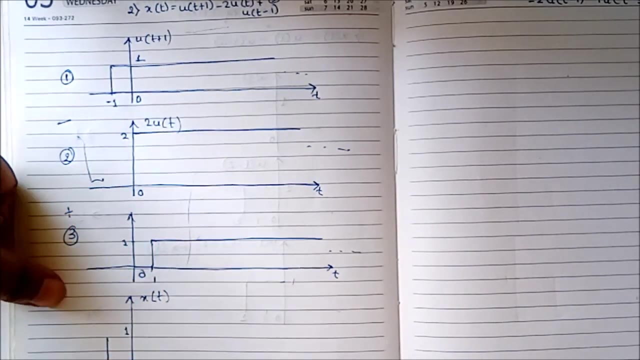 At 0, the first signal's amplitude is 1.. Second signal's amplitude is 2.. And third signal's amplitude is 0.. So minus 2 is minus 1 plus 0.. So it is minus 1.. So we will draw that signal. 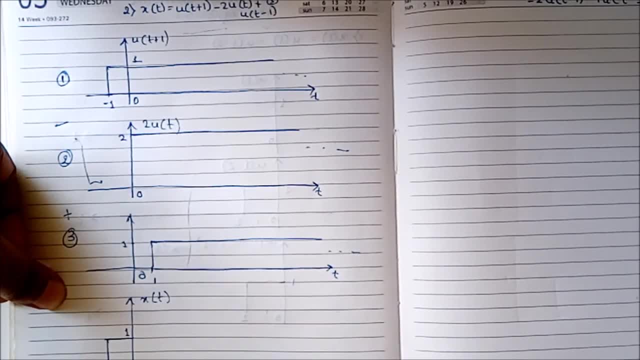 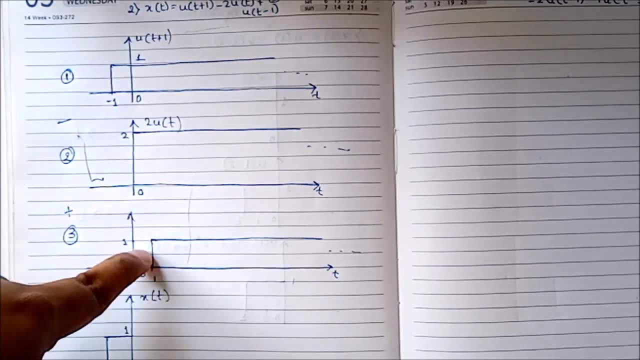 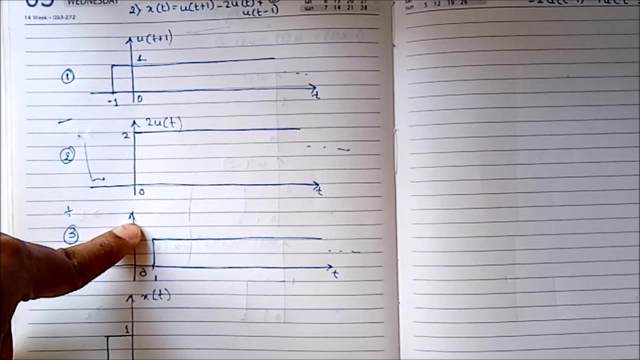 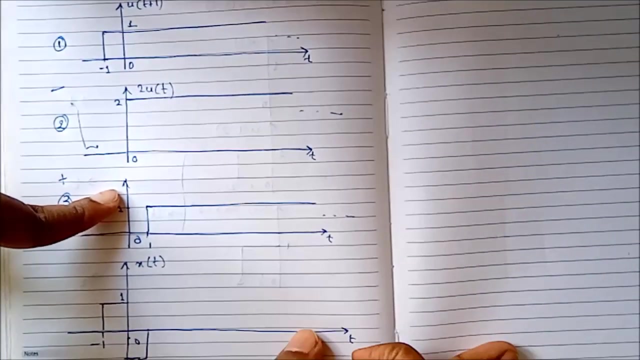 At 1 the first signal's amplitude is 1, second signal's amplitude is 2 and third signal's amplitude is 1.. So 1 minus 2 is minus 1.. Minus 1 plus 1 is 0.. So at 1 the signal is again going to go back to 0.. 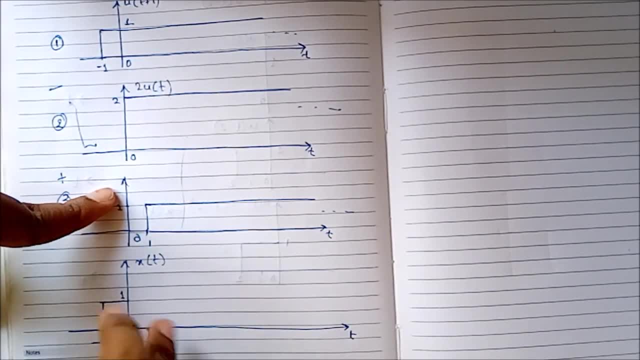 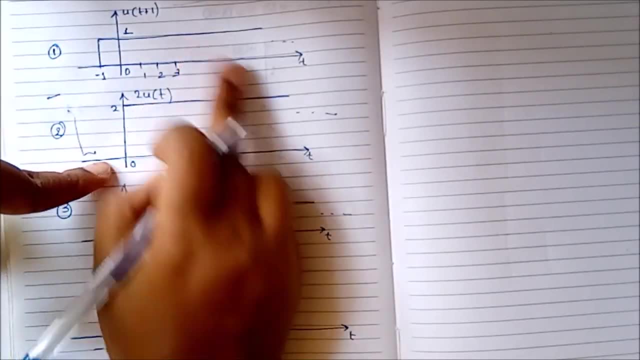 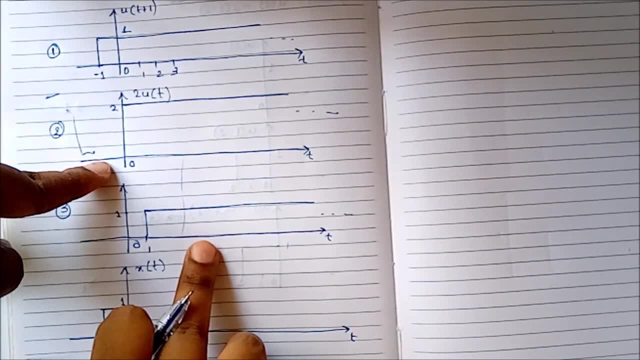 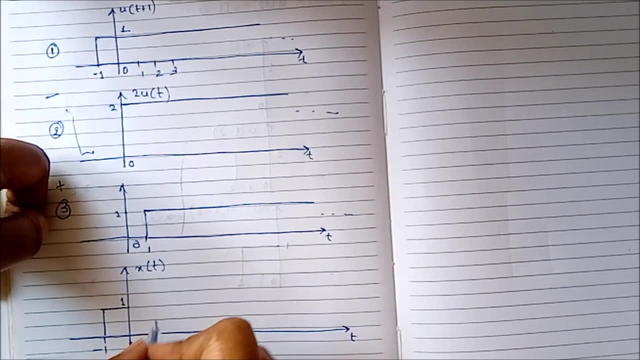 The second signal's amplitude is 2 and the third signal's amplitude is 1.. So 1 minus 2 is minus 1.. Minus 1 plus 1 is 0.. So after 1 on the t-axis, all the points are going to be 0.. 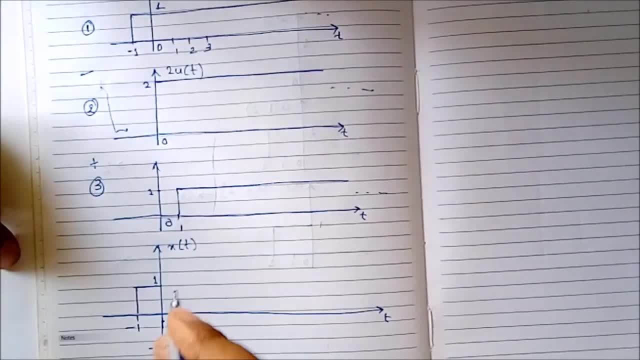 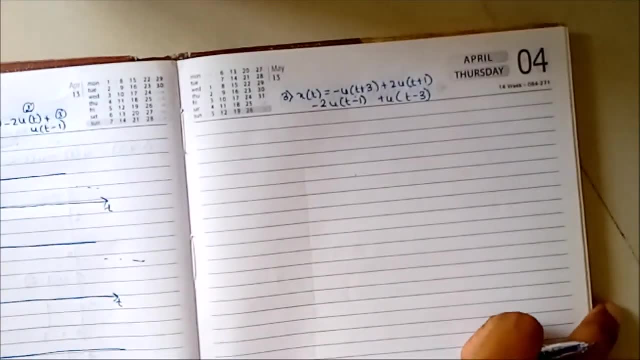 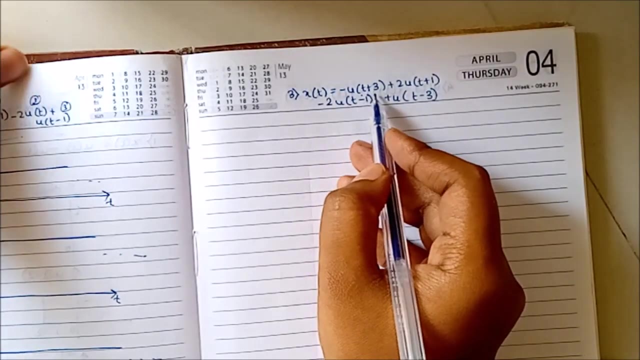 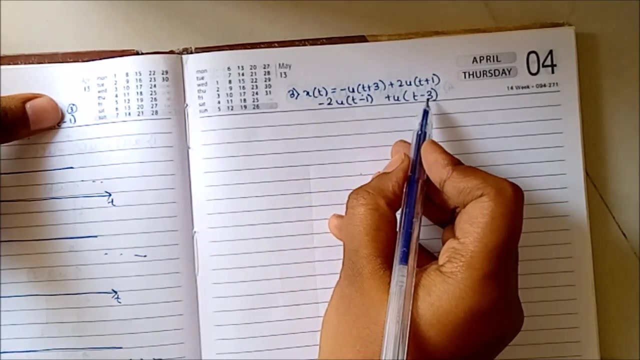 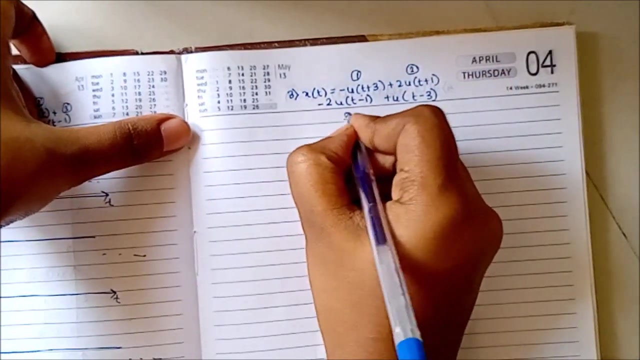 So this is the resultant signal which we required, which is x of t. Now the third question. x of t is equal to minus u of t plus 3 plus 2, u of t plus 1 minus 2, u of t minus 1 plus u of t minus 3.. This is the first signal, second, third and fourth. 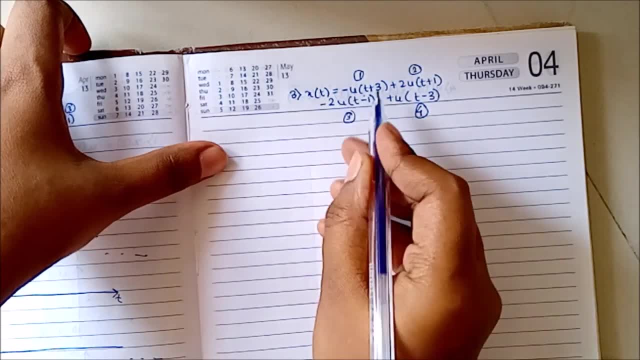 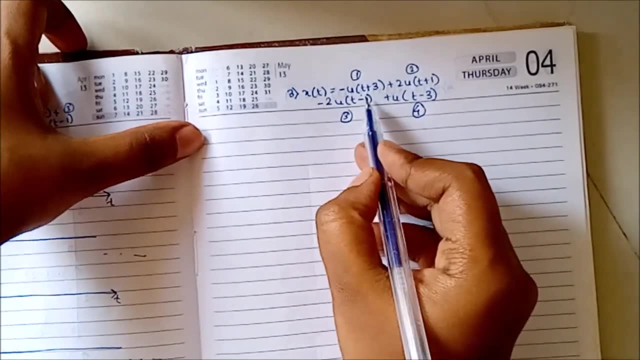 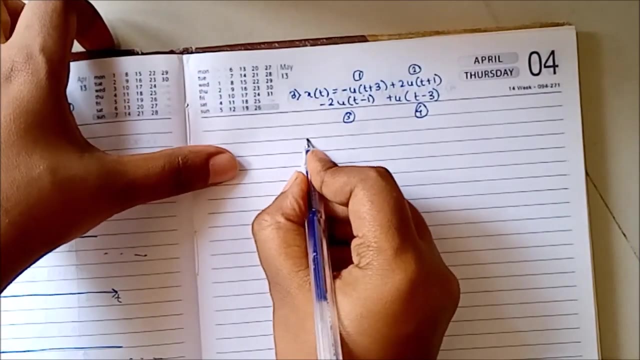 Now here for the first signal. we have a minus sign, So we will have to just draw it on the opposite side of the t-axis. It's an advanced version of the unit step signal by 3, and then we have to negate it. So this is the t-axis. 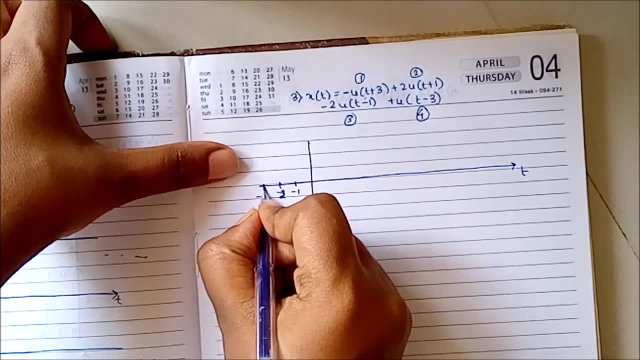 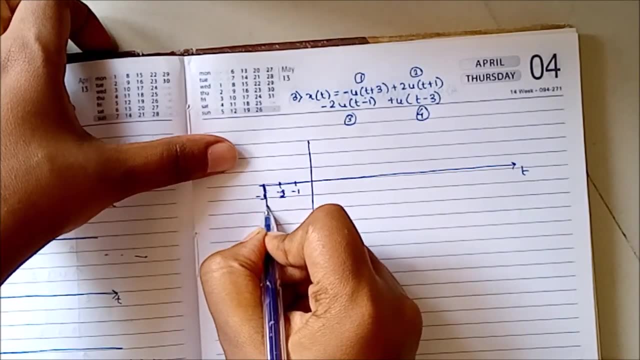 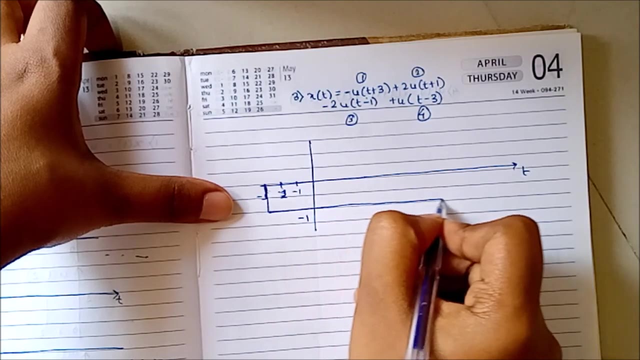 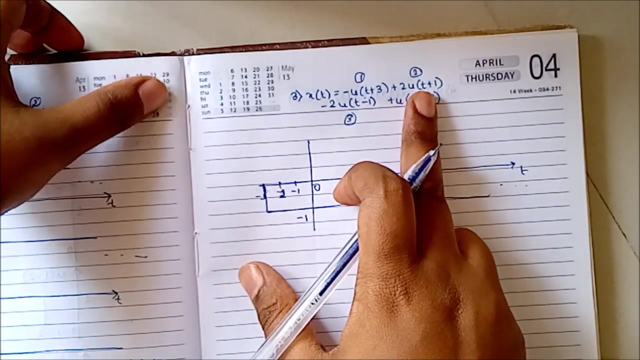 And the signal is b. So this is the beginning at minus 3. but it will be the negated version of the unit step signal, So the amplitude will be at minus 1.. So this will be the signal. Now for the second signal. this is an advanced version of the unit step by 1 multiplied by 2.. 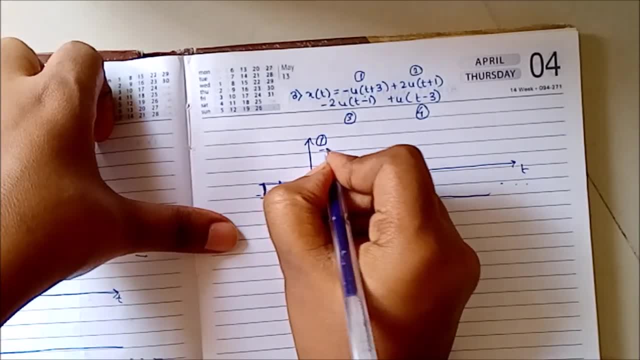 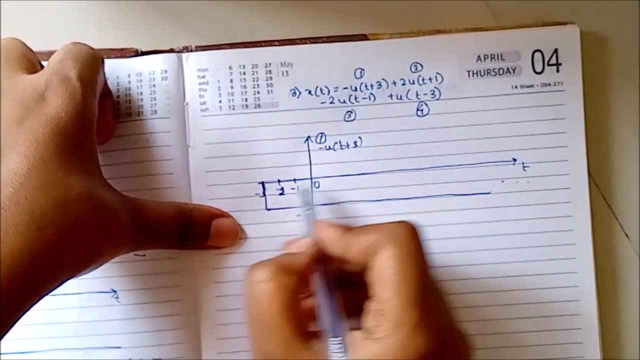 So this is the first signal. So this is the second signal. So this is the first signal. So this is the first one Minus u of t plus 3.. We can also subtract the first signal instead of drawing it in the negated manner. 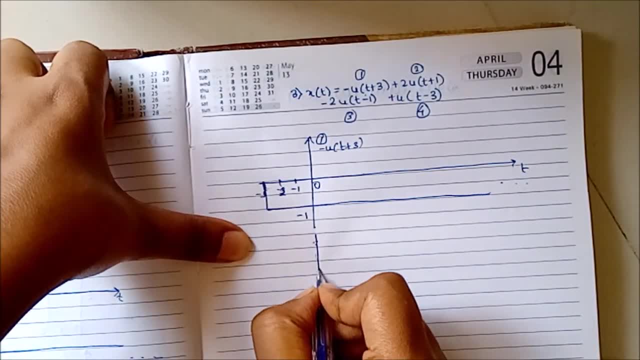 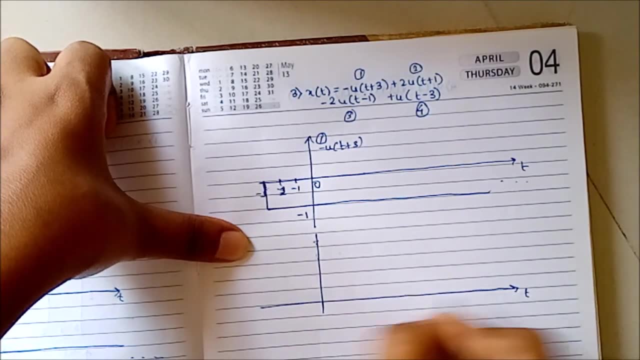 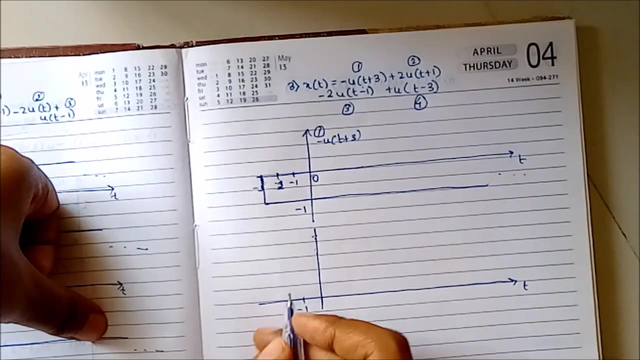 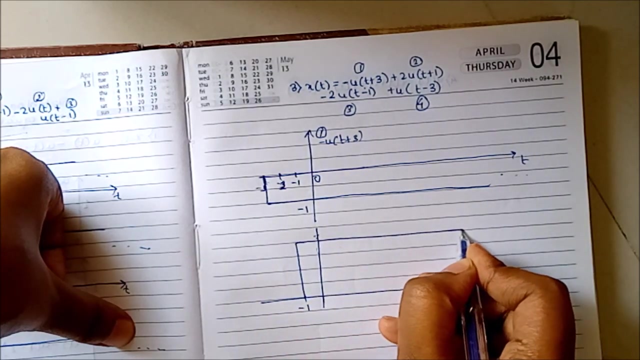 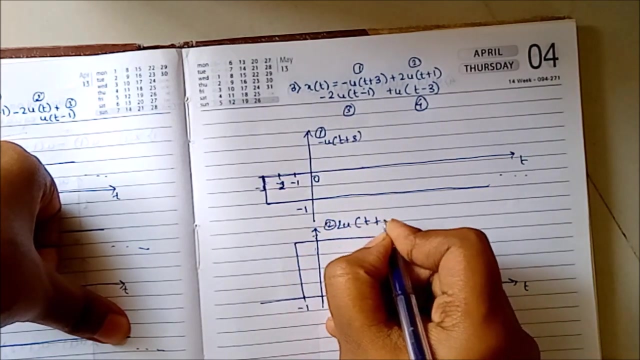 But this will make our work easier. Now the second signal will have amplitude of 2.. So it will start at minus 1.. So it will start at minus 1 with amplitude 2.. So this is the second one: u of t, 2u of t plus 1.. 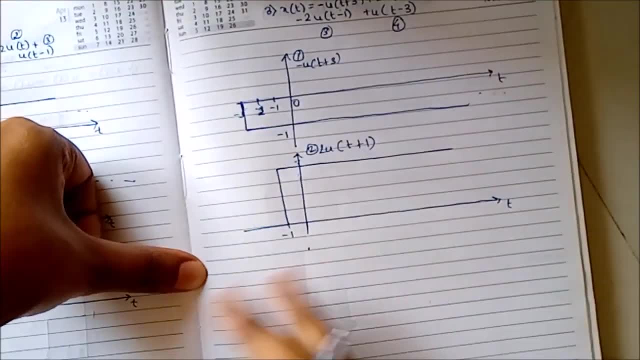 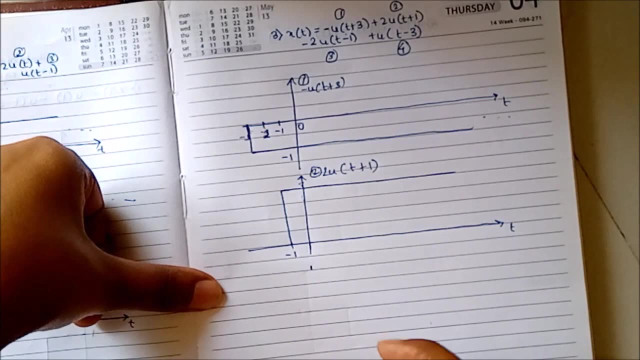 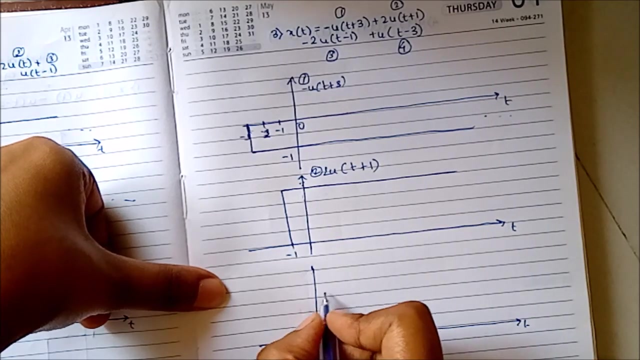 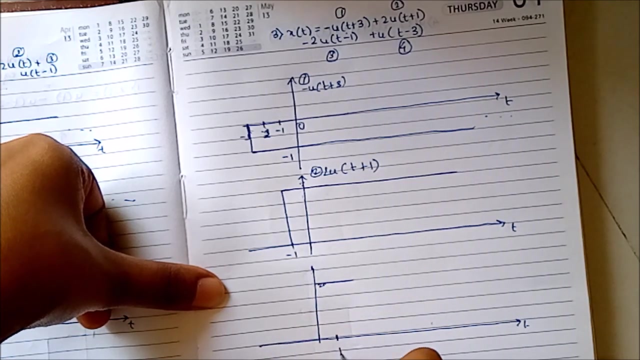 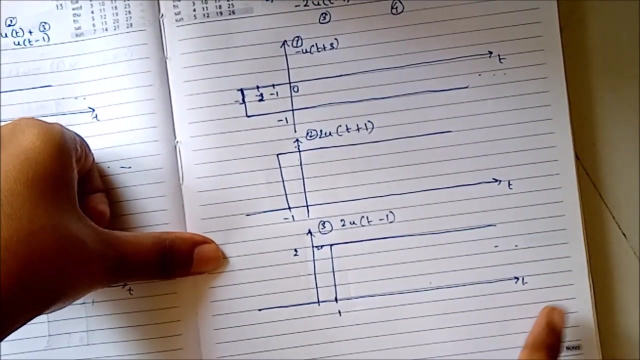 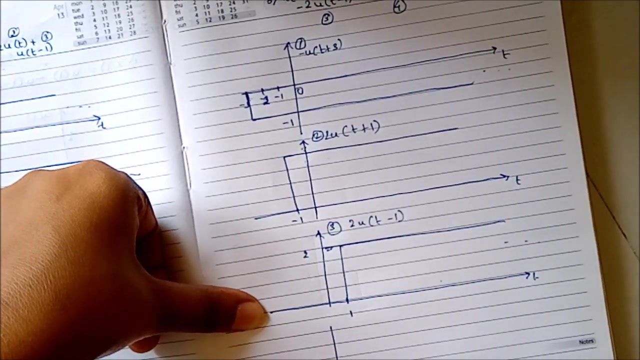 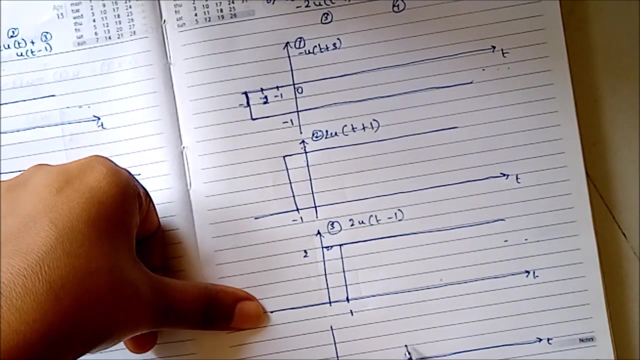 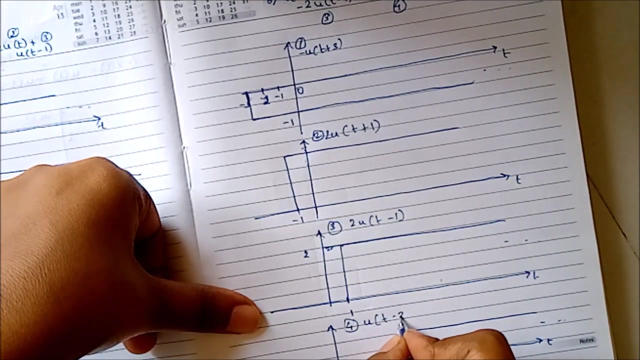 The third signal is minus 2u of t minus 1.. And this is the delayed version with amplitude 2.. So this is the delayed version with amplitude 2.. This is the fourth one: u of t minus 3.. Now we have to add the first with the second. 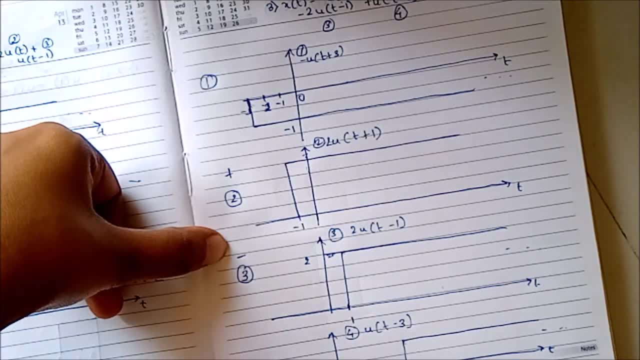 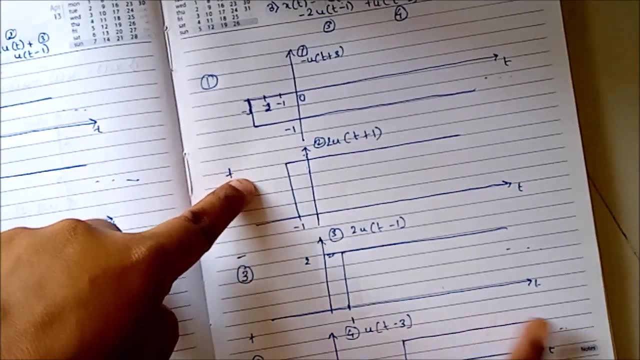 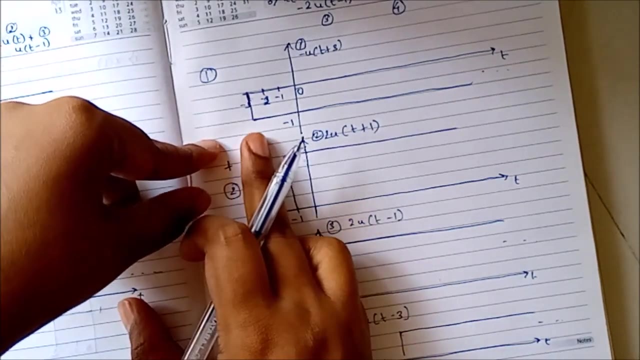 And then subtract it with the third And then add it to the fourth. So our first signal is starting at minus 3.. The rest are all beginning from the next point. So we can consider minus 3 as our first point for the resultant. 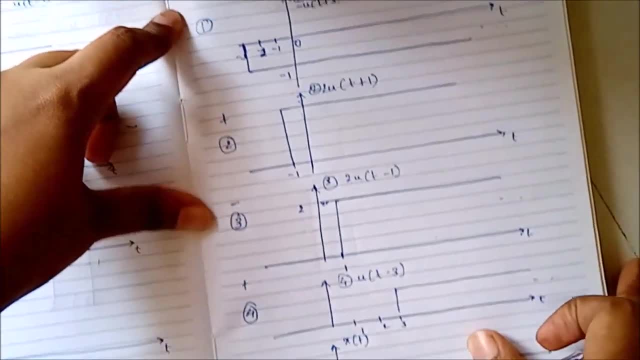 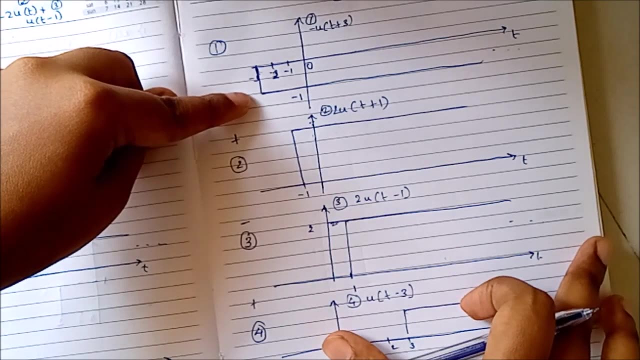 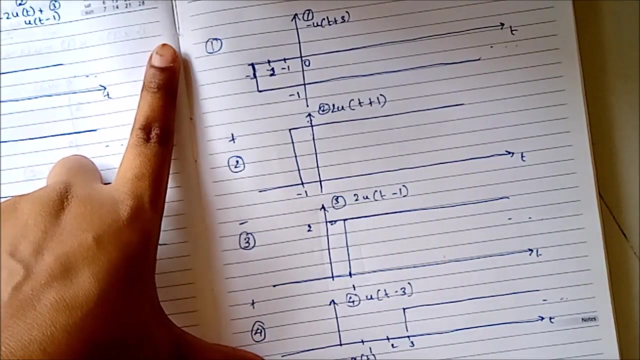 This is x of t. Now we are adding the second one, Adding the first, So the amplitude is minus 1.. Minus 1 plus 0.. Minus 0 plus 0.. So the resultant amplitude is minus 1.. 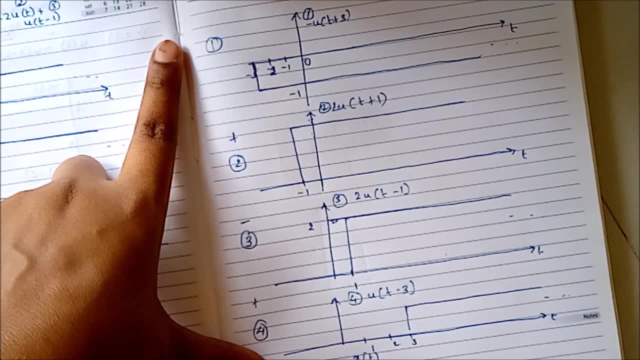 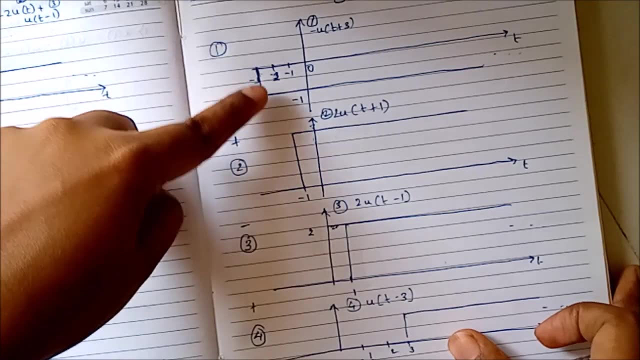 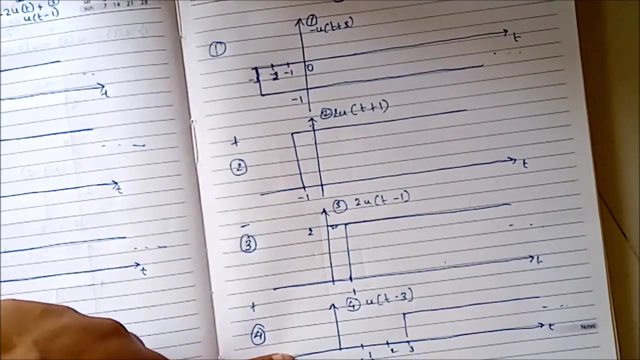 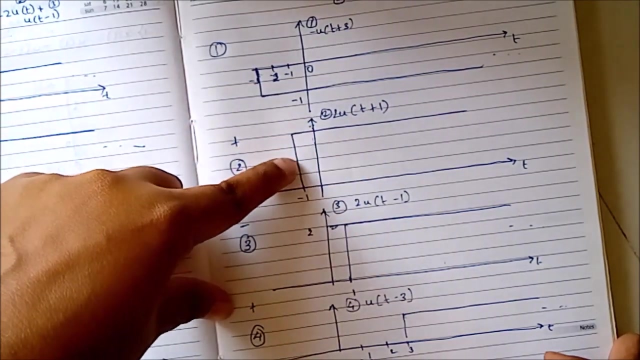 At minus 3.. At minus 2.. The amplitude is again minus 1 plus 0.. Minus 0 plus 0.. So again minus 1.. At minus 1, minus 1 plus 2. So that is 1.. 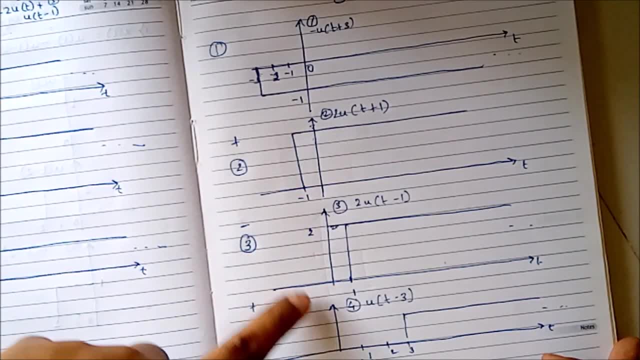 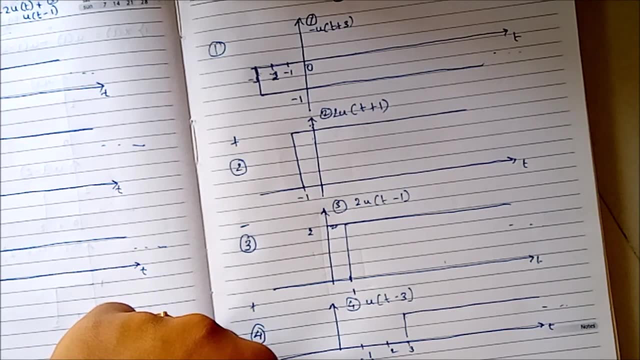 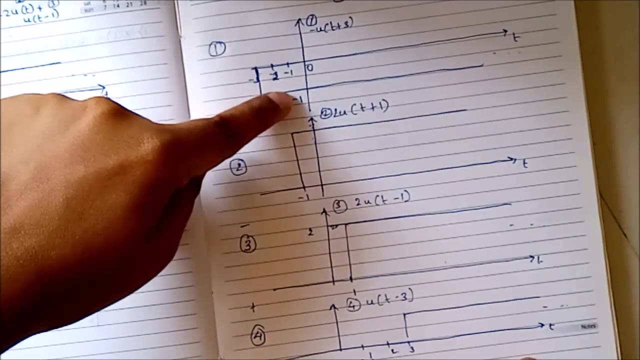 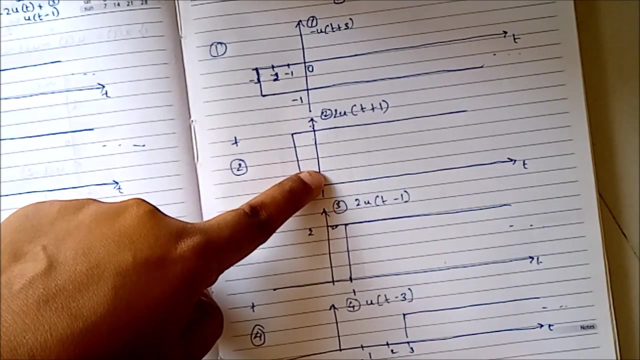 1 minus 0 is 1. And then plus 0 is 1.. So the amplitude is going to be plus 1 and minus 1.. At 0 the amplitude is minus 1, minus 1 plus 2 is 1, 1 minus 0 is 1, 1 plus 0 is again. 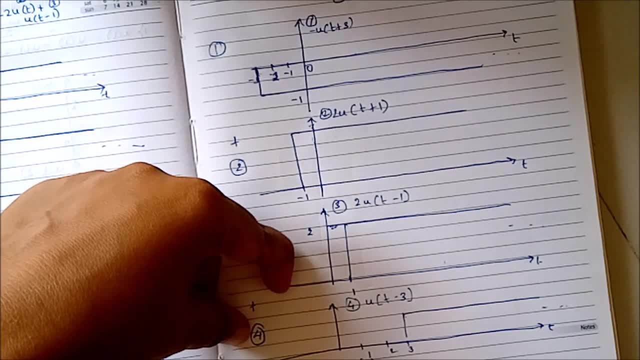 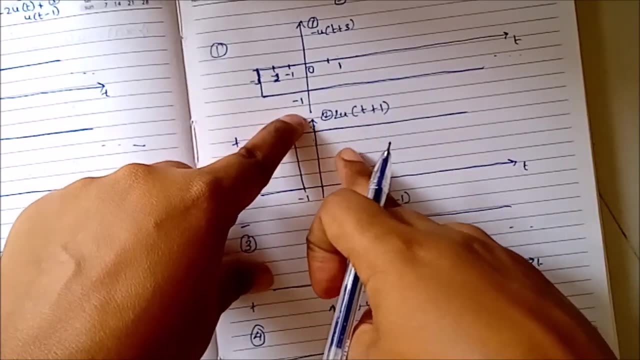 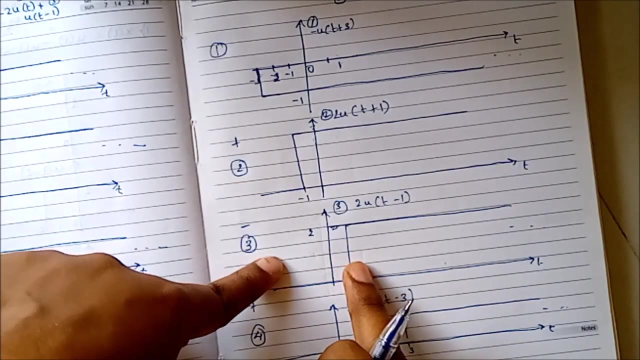 1. So the amplitude is 1. At 1, the first signal's amplitude is minus 1, second is 2. So minus 1 plus 2 is 1, 1 minus 2 is minus 1, minus 1 plus 0 is minus 1. So this signal is going. 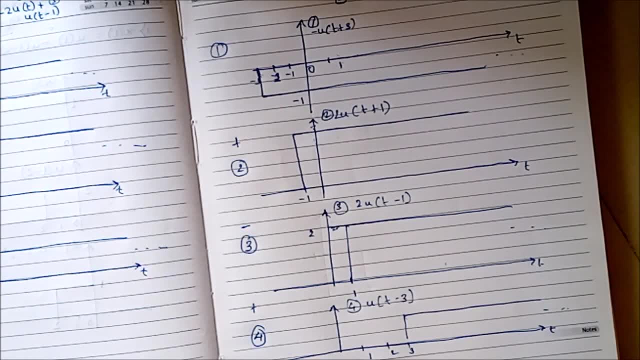 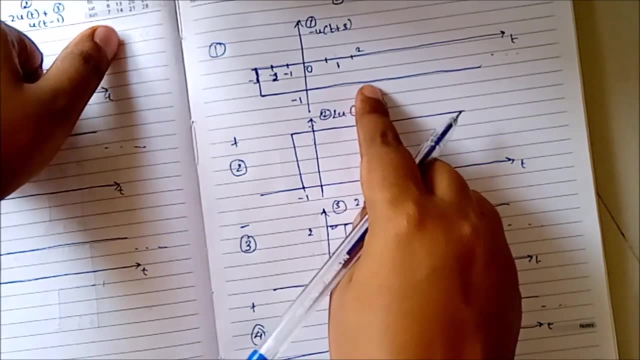 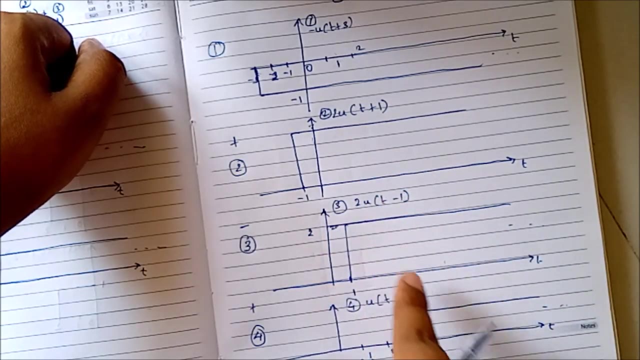 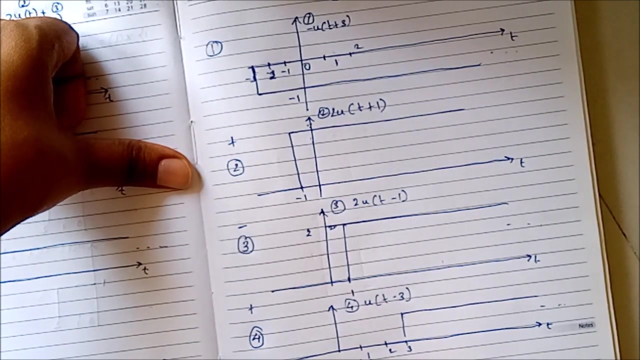 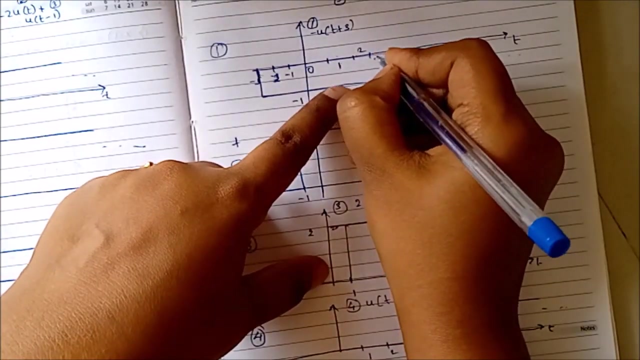 to minus 1.. At 2, the first signal's amplitude is minus 1, minus 1 plus 2 is 1, 1 minus 2 is minus 1, minus 1 plus 0 is again minus 1.. At 3, the first signal's amplitude is minus 1, minus. 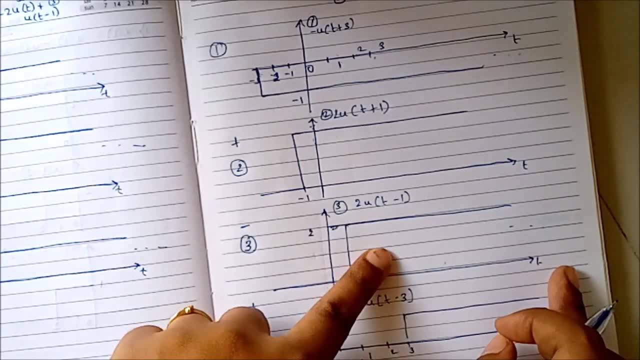 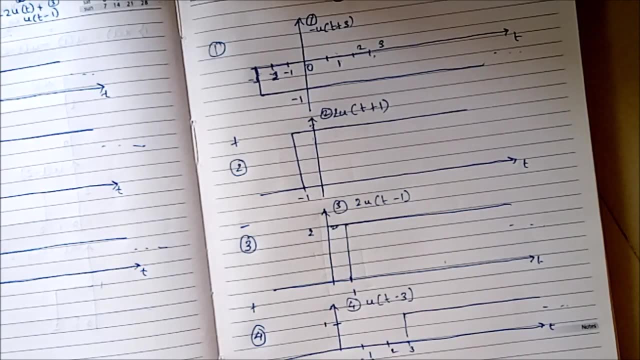 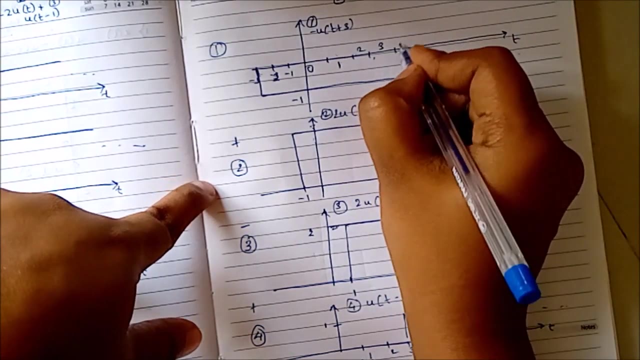 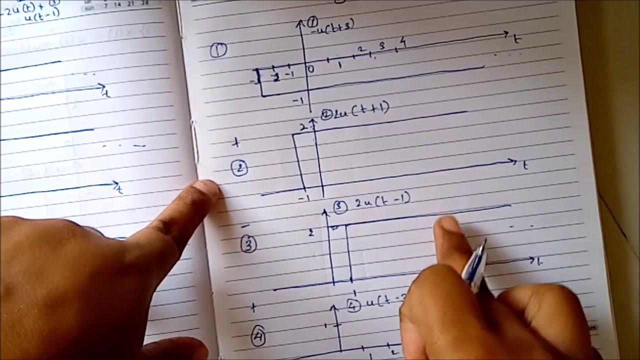 1 plus 2 is 1, 1 minus 2 is minus 1, minus 1 plus 1 is 0. So the signal goes back to 0 at 3.. At 4, the first signal's amplitude is minus 1, minus 1 plus 2 is 1, 1 minus 2 is minus. 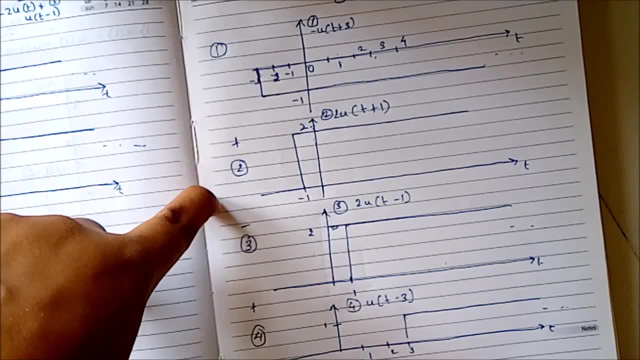 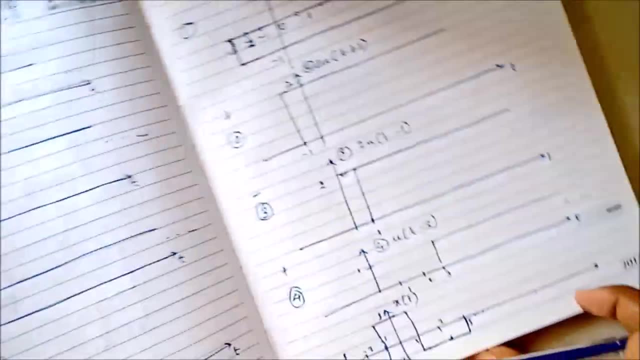 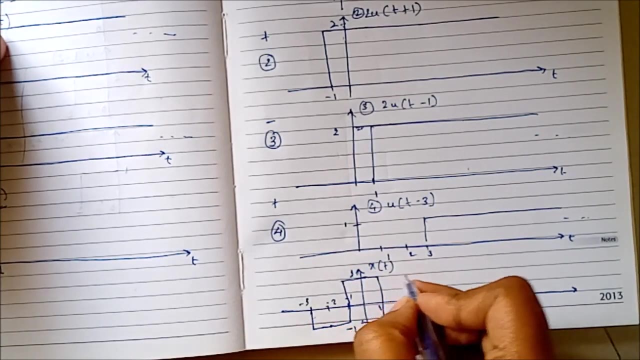 1, minus 1 plus 1 is 0.. So this is the first signal's amplitude. So the rest, all these points, are going to be zeros. So this is the resultant signal which we have got. So here is the result of x, of t. It's a symmetric signal about the 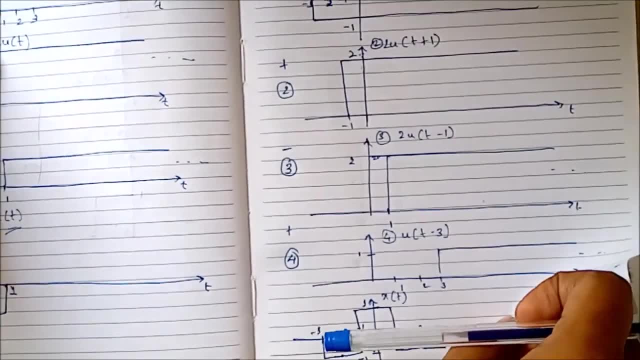 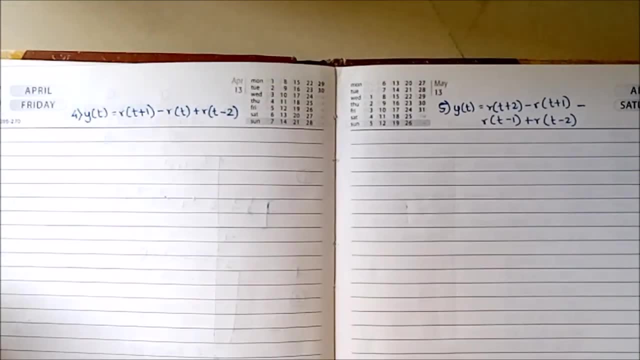 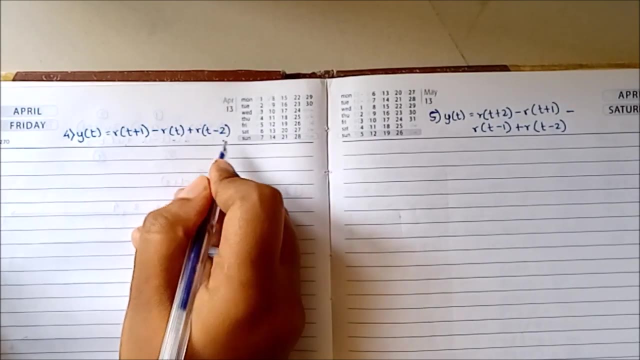 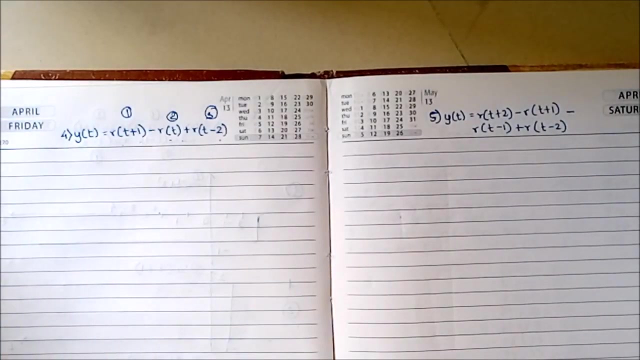 vertical axis. Now we will go to the next example. This is a ramp type of question. So here we have r of t plus 1, r of t and r of t minus 2.. So let's name them first, second and third. 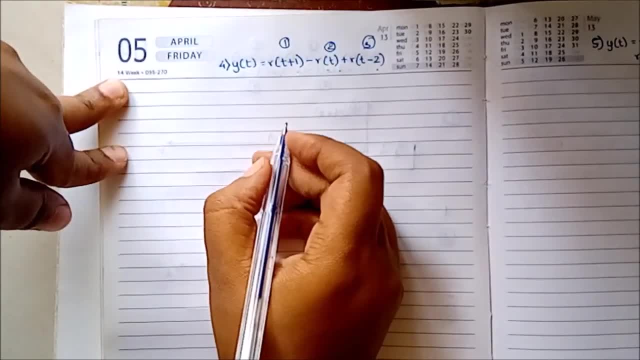 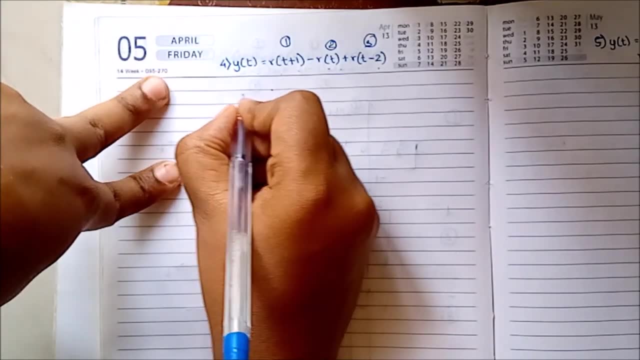 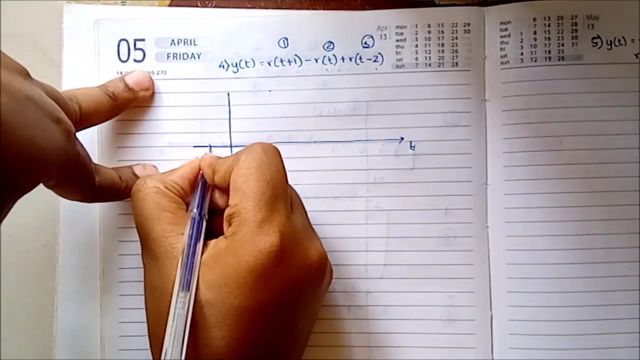 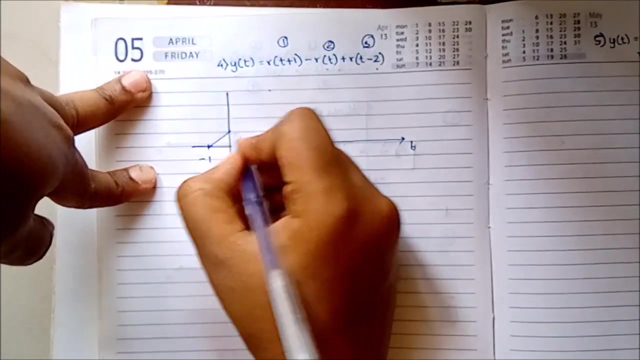 Let's draw the first signal. So r of t plus 1 is the advanced version of the unit ramp signal by 1.. So let's draw it So it will begin at minus 1.. At 0, the amplitude will be 1, at 1, the amplitude will be 2, at 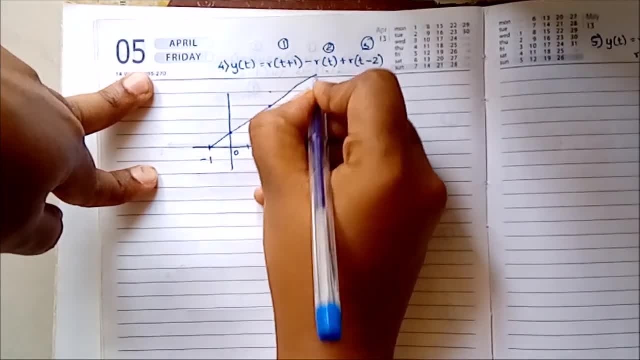 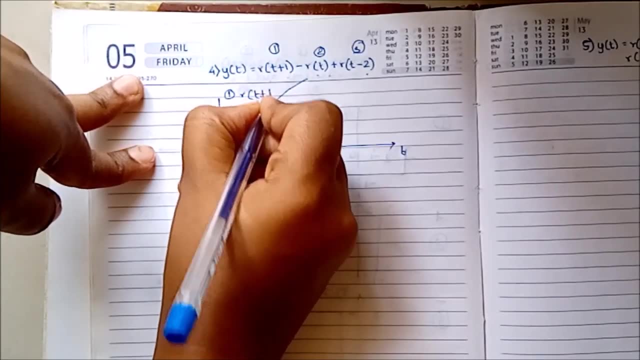 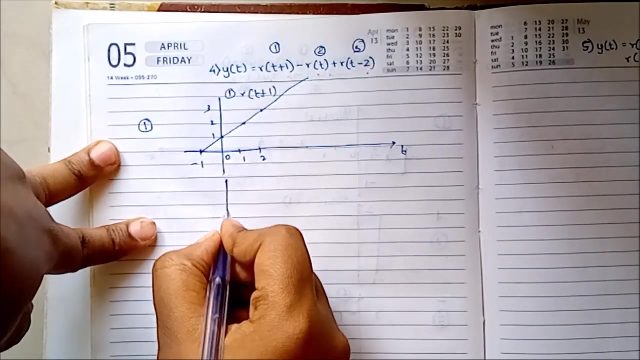 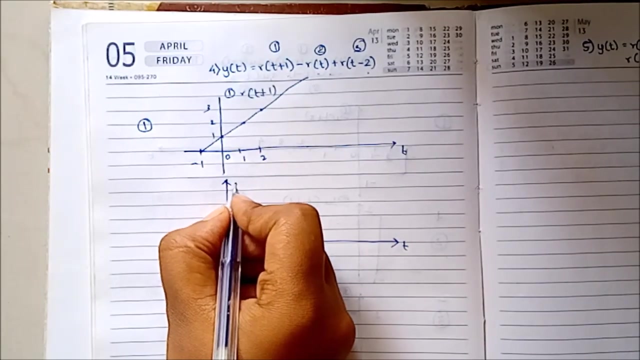 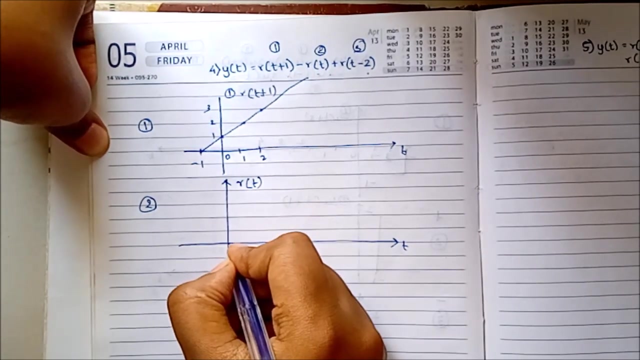 2, the amplitude will be 3, and so on. So this is the first one, that is r of t plus 1.. Second signal is r of t, So this is the usual unit ramp. This is where f of t is the master champion. Second signal is r of t, as it is, So the first. 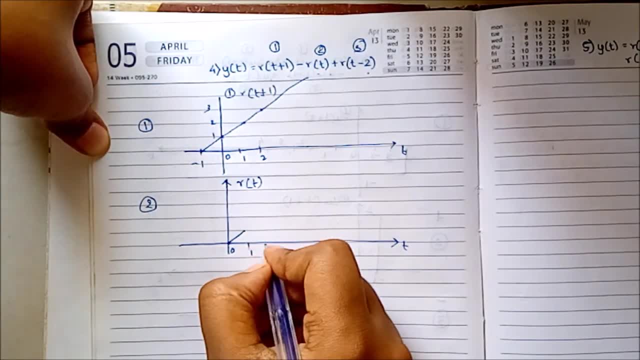 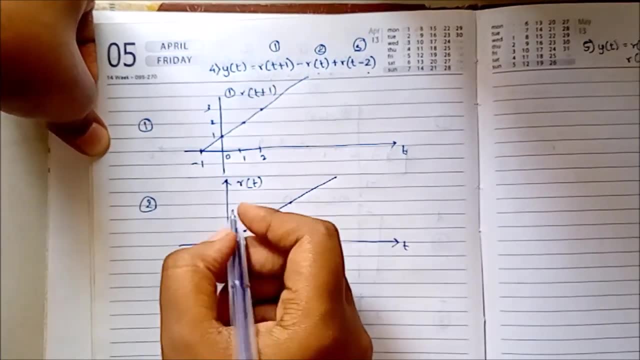 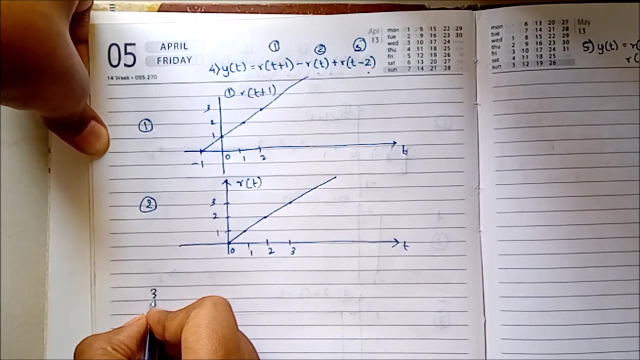 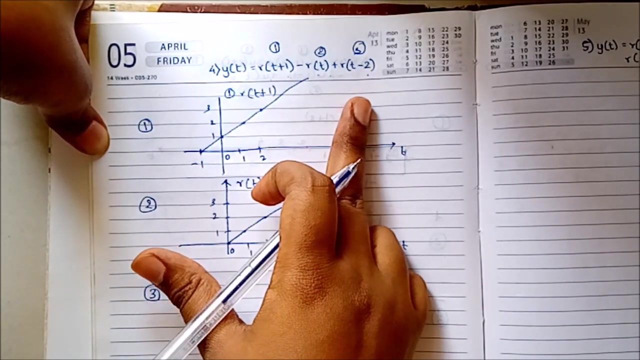 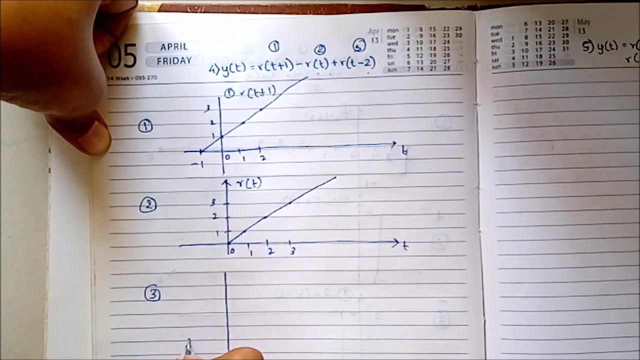 signal culture is r of t plus 1.. So let's choose master y, which is the ramp type, and this is r of t plus 1, as seen here For extraכ f land band r. Now lets draw the third signal. The third signal is R, so this is a delayed version of the unit ramp by 2.. 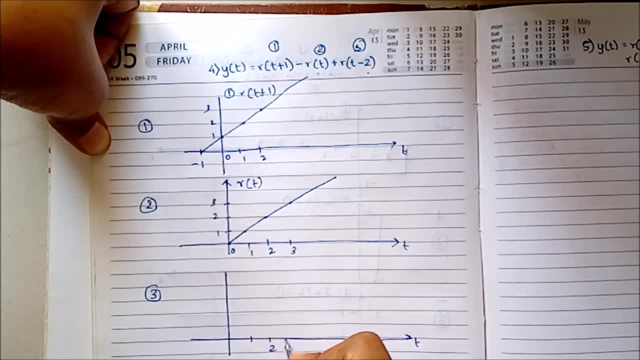 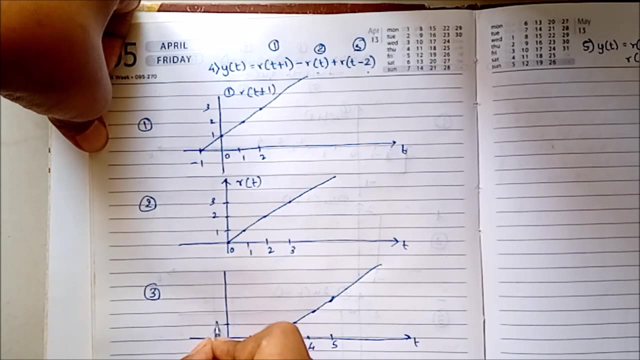 So it will begin at 2.. At 2, the amplitude will be 0, at 3, the amplitude will be 1, at 4 the amplitude will be 2, at 5 the amplitude will be 3, and so on. 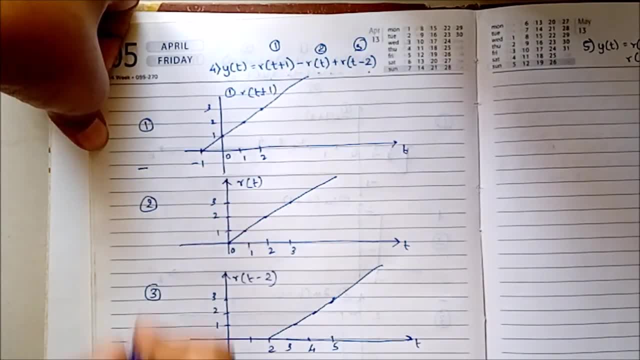 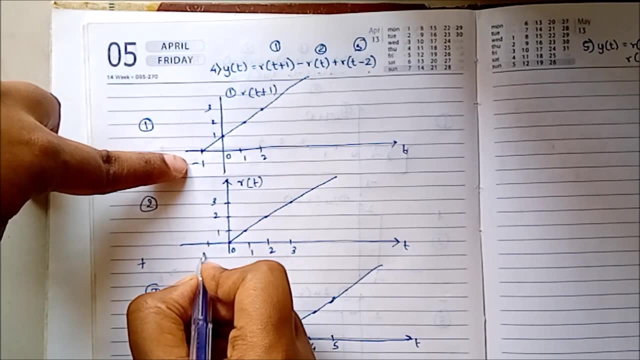 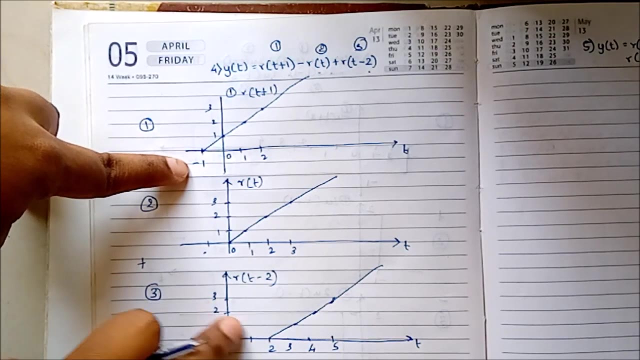 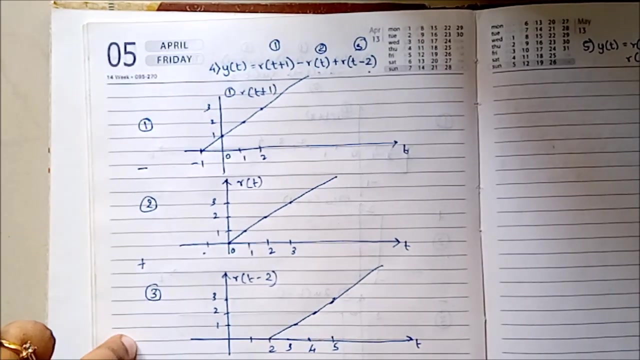 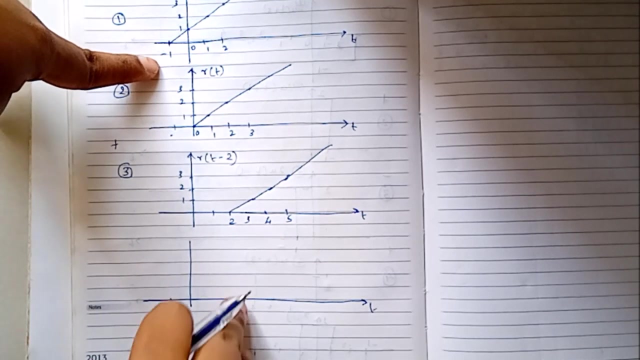 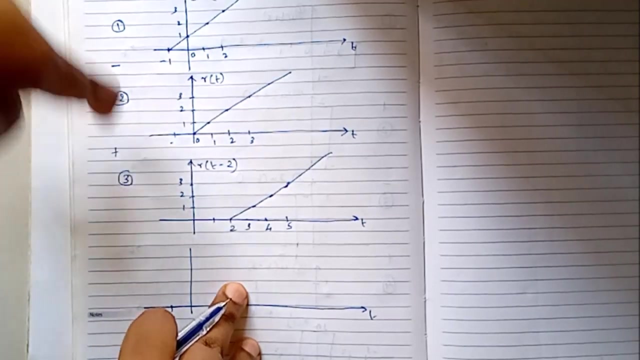 Now we have to subtract the second signal from the first and then add the third one. So lets start The signal which is starting. the first is the first one itself. Now, at the first signals, amplitude is 0,. second signal, amplitude is 0 and third is: 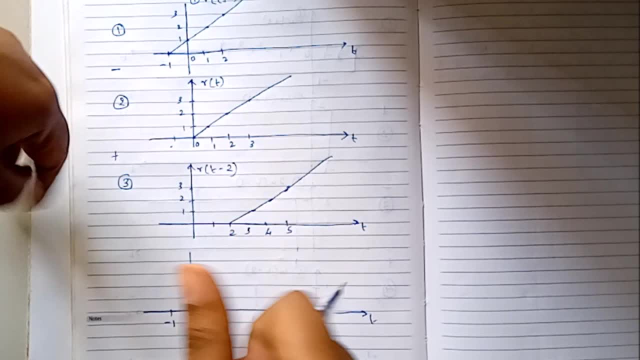 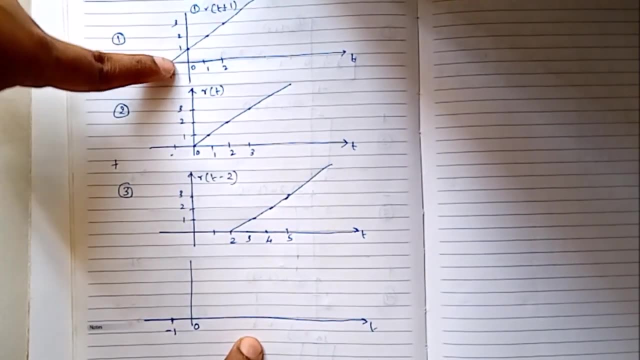 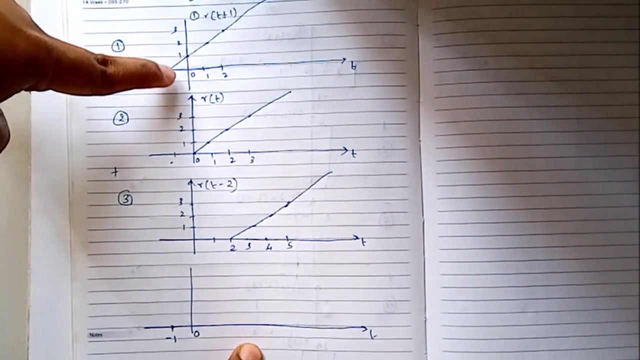 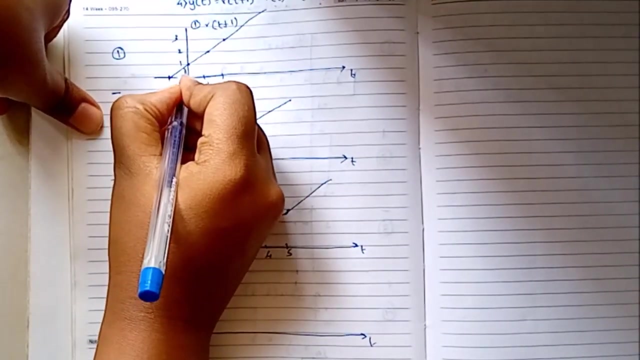 also 0.. so zero minus zero plus zero is zero. so here we don't have any amplitude at zero. the first signal's amplitude is one, second signal's amplitude is zero and third signal's amplitude is zero. so it will be one minus zero plus zero, so one. and because this is a triangular, 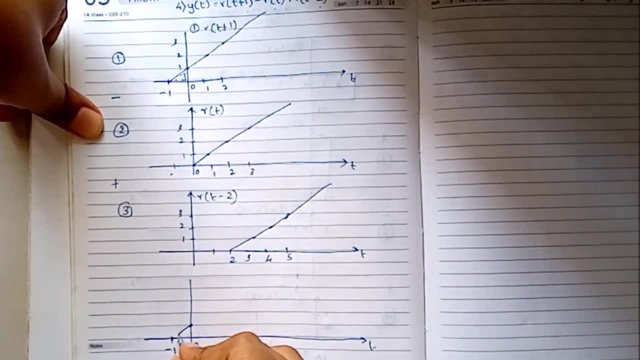 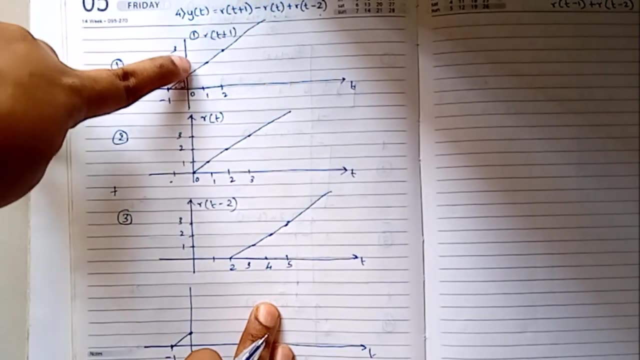 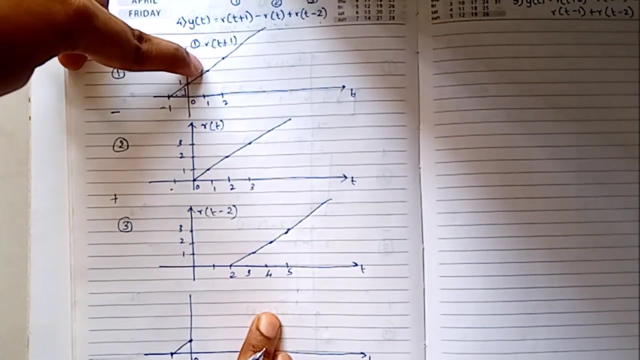 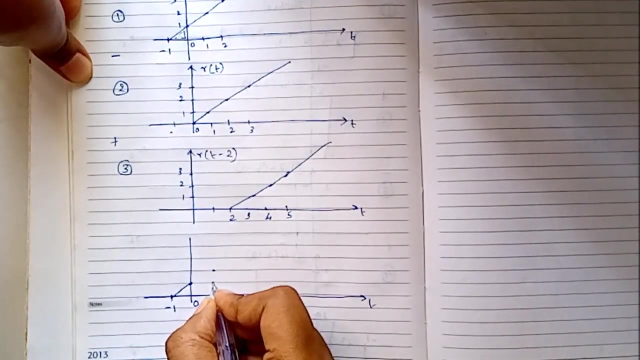 or ramp shaped signal. here also it will be representing a ramp now at one. the first signal's amplitude is two, the second signal's amplitude is one and third signal's amplitude is zero. so two minus one plus zero is one. so it will be amplitude as one here and we can see that. 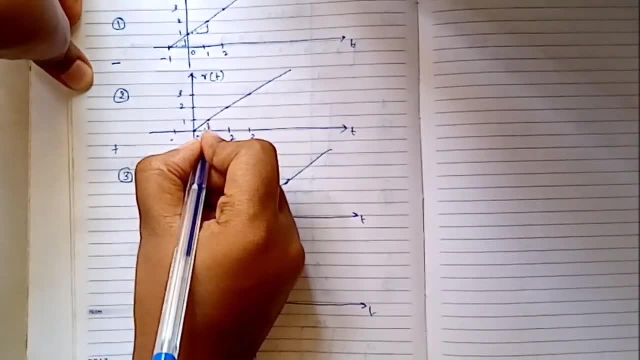 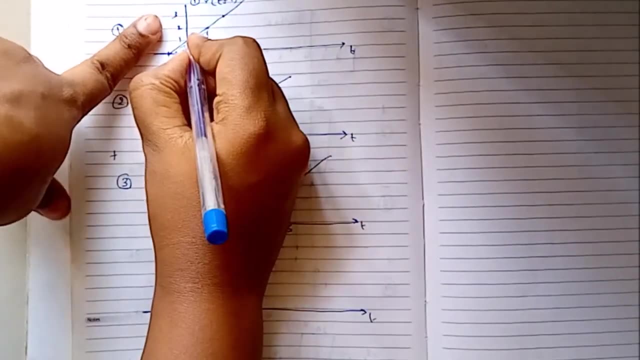 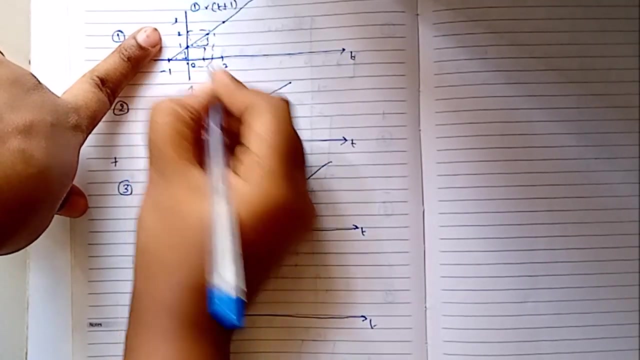 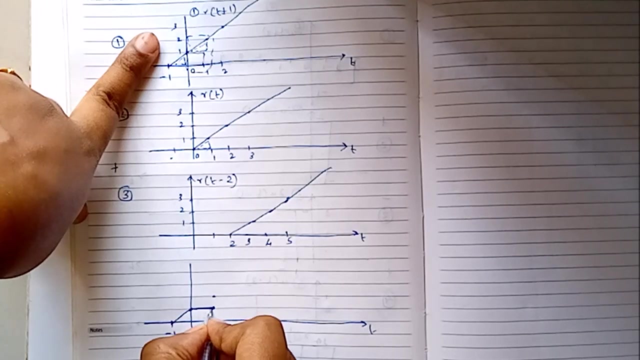 this triangular part is also there in the second signal, and the second signal's triangular part is getting subtracted from the first signals- this portion, first portion- so in the resultant signal we'll only have the rectangular shape. so here the signal will be of a step signal and not a ramp. 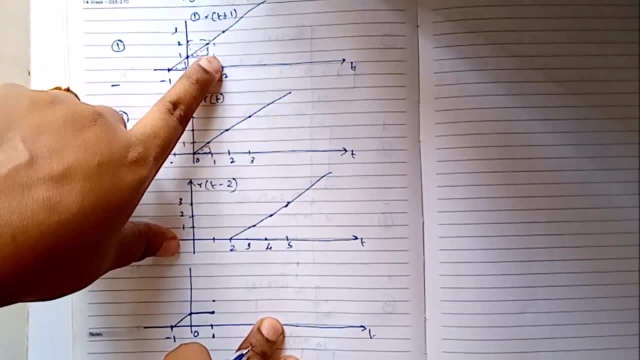 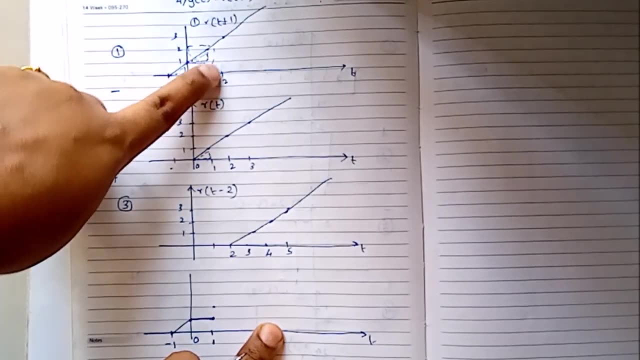 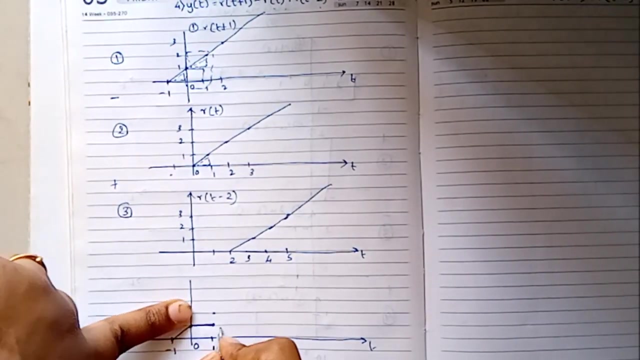 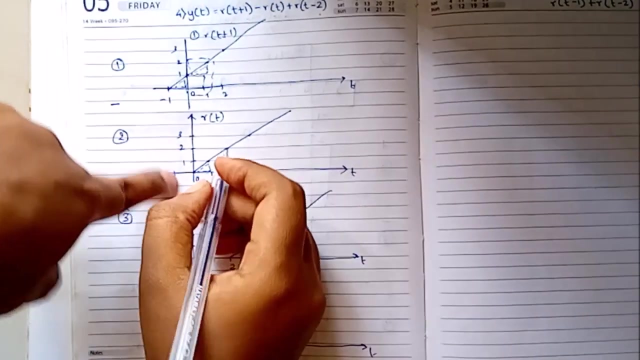 at two. the first signal's amplitude is three, second signal's amplitude is two, and first the third signal's amplitude is zero. so three minus two is one, one plus zero is one. so again the amplitude is going to be one at two. so the same, uh, the same step is going to apply, because here there's a ramp. 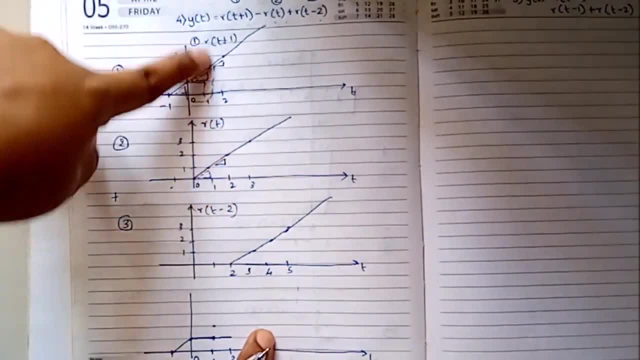 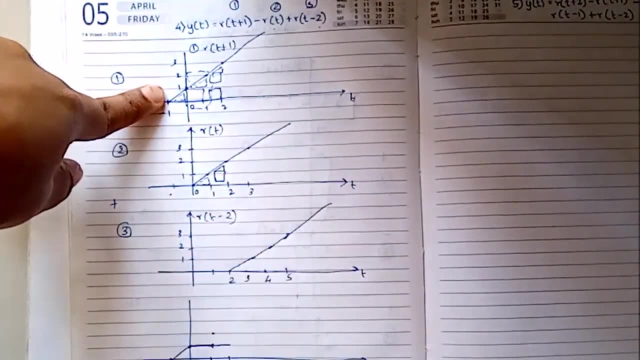 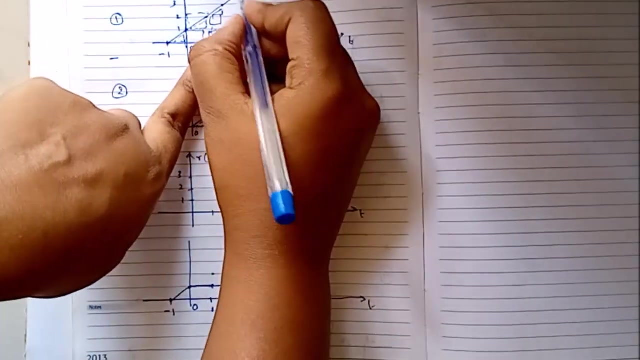 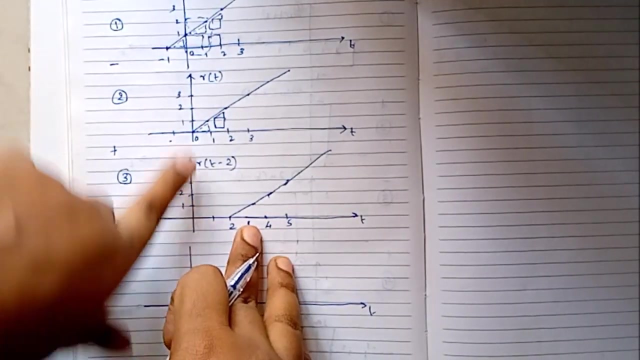 and here there is a ramp, so this ramp is getting deleted. so here there is a gap. the shape is getting deleted from here, so we only this step is remaining at at three. the first signal's amplitude is four, the second signal's amplitude is three and the third signal's amplitude is one. 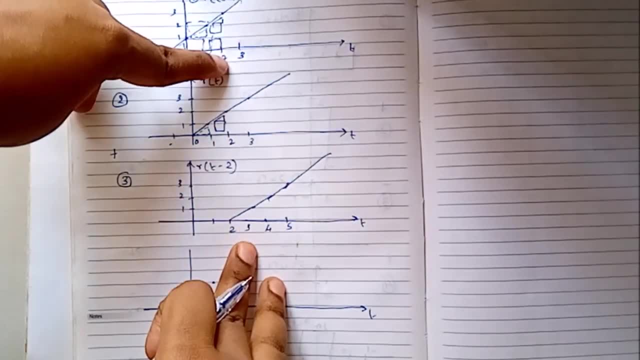 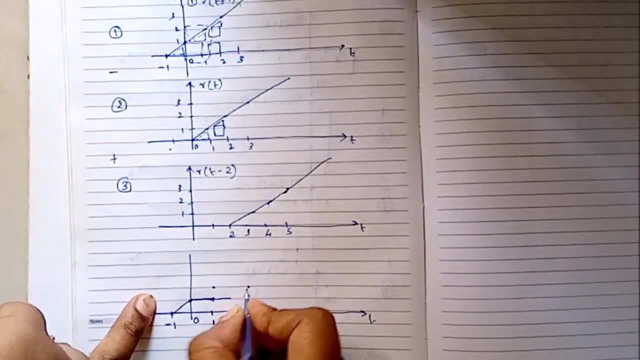 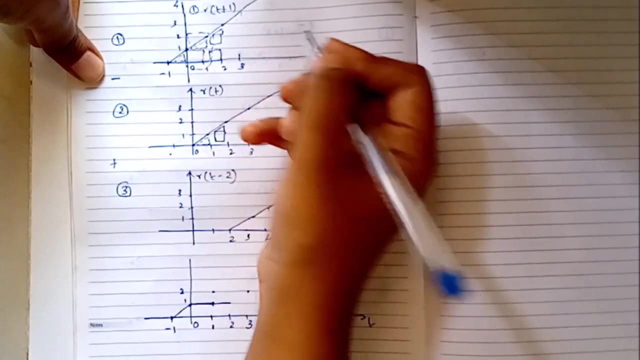 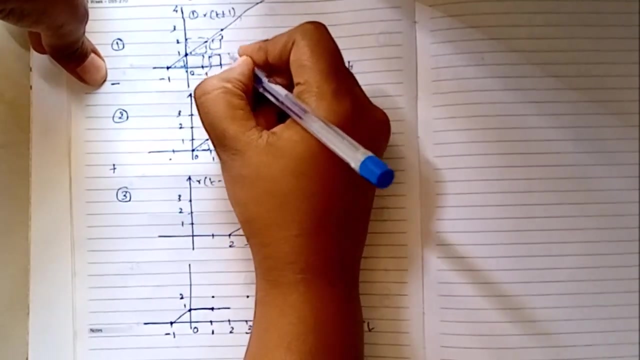 four minus three is one and one plus one is two. at this point, at 3, our amplitude is going to be 2 and if we see the signal from the first signal, this much portion is going to get minus. so how much is going to remain is? 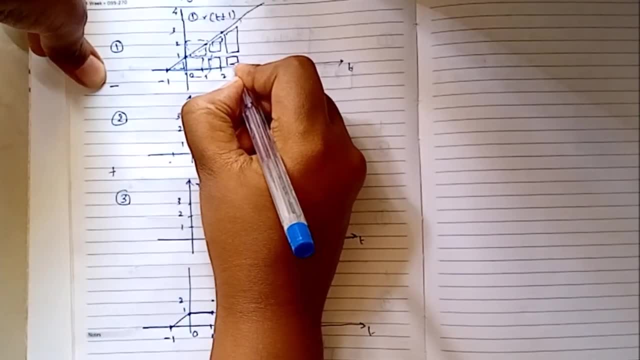 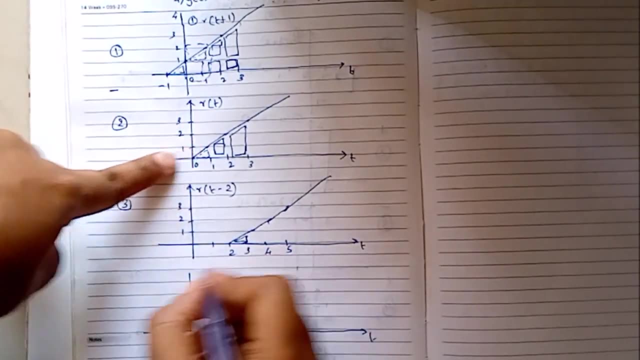 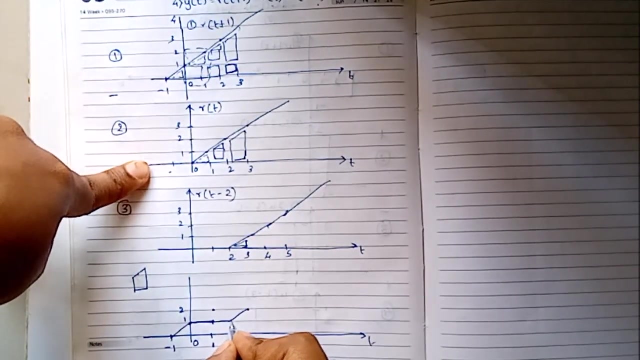 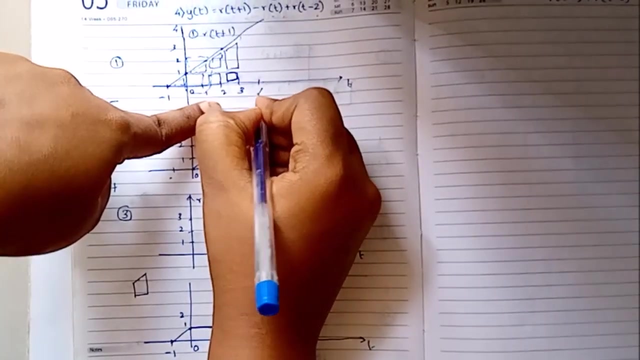 is this step, and this step is going to get added to this ramp. so we are going to get a shape like this here. so it is going to be something like this: at 4, the first signal's amplitude is 5, the second signal's amplitude is 4 and the third 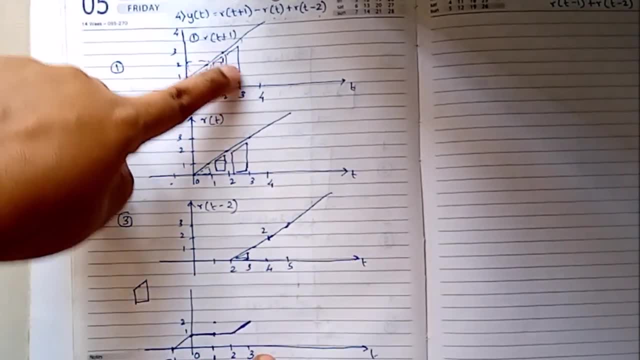 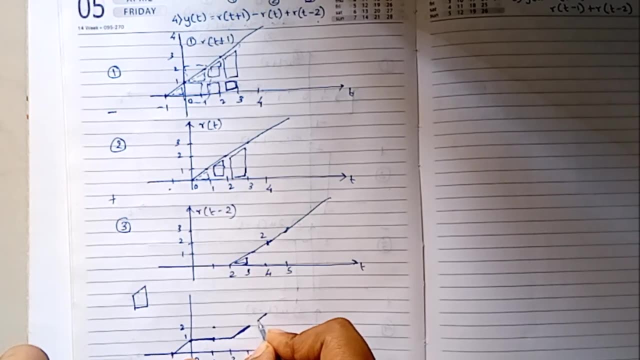 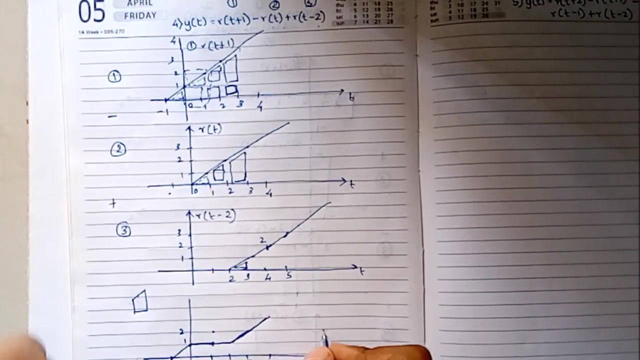 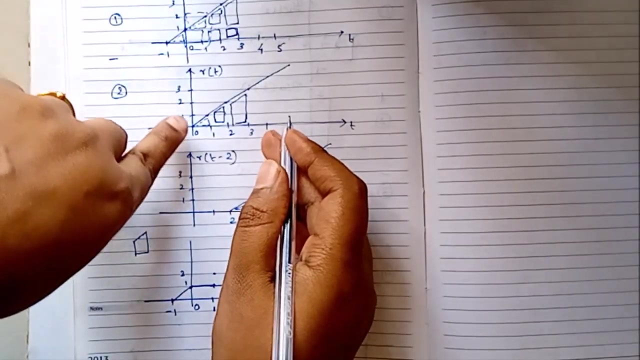 signal's amplitude is 2, so 5 minus 4 is 1. 1 plus 2 is 3, so this is going to continue to 3 and it is going to follow the same logic as the previous step we used at 5. the first signal's amplitude is 6. the second signal's amplitude is 5, so 6 minus. 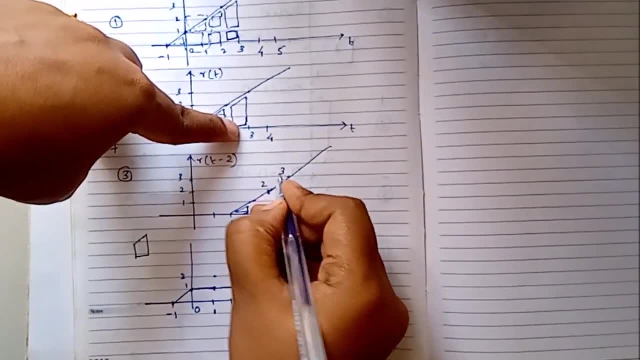 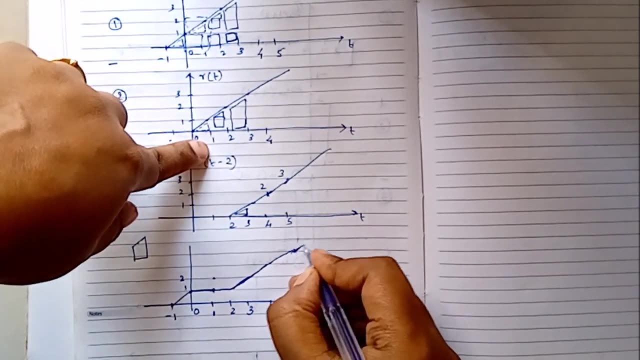 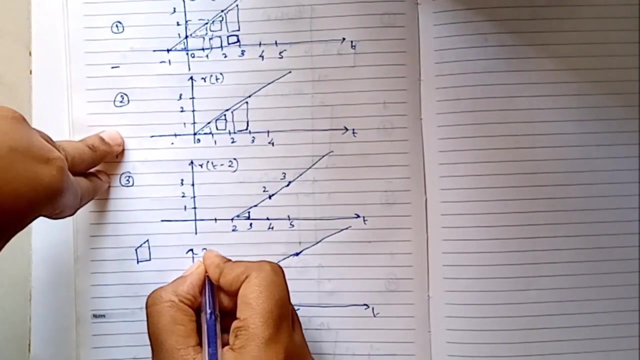 5 is 1 and 1 plus 3, so it is going to be 4, following the same step, and this is going to continue till the end, because the shapes of the signals are constant. so this is the result in x of t which we require. 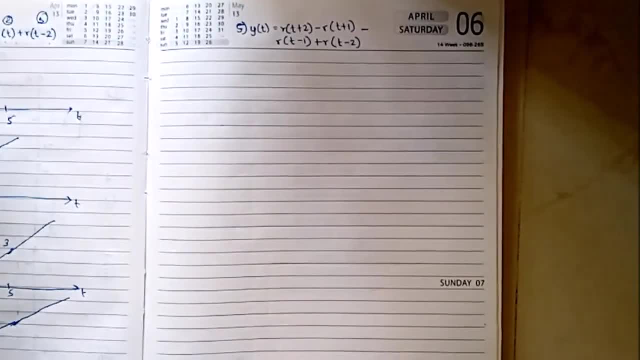 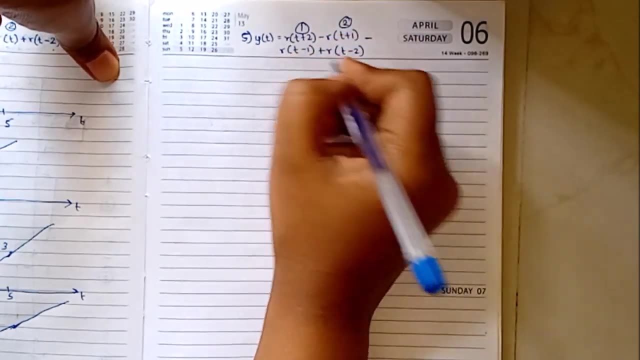 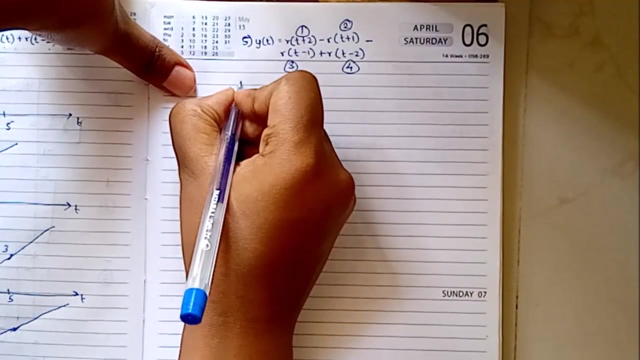 now we will solve one more sum in which we are using ramp signals. so here we have the first signal as r of t plus 2, second as r of t plus 1, third as r of t minus 1 and fourth as r of t minus 2. so let's draw the first signal. 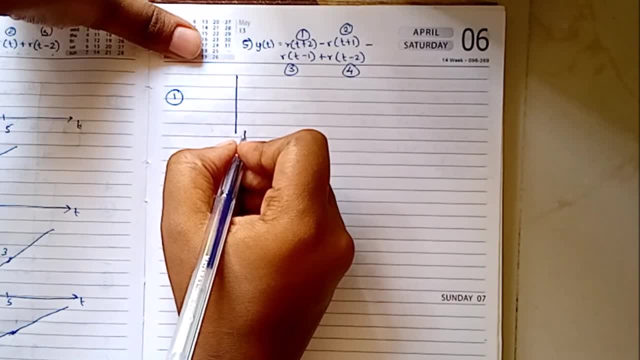 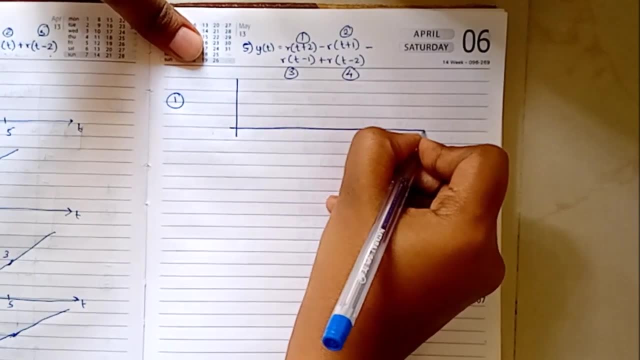 so here we are using for the first time r of t as 1, followed by r of 1 of 2 and r of r of 3, which are same values. as for r of 1 and r of 2 we are using for initial. 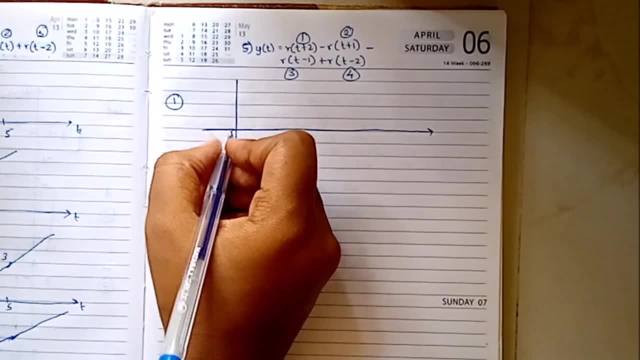 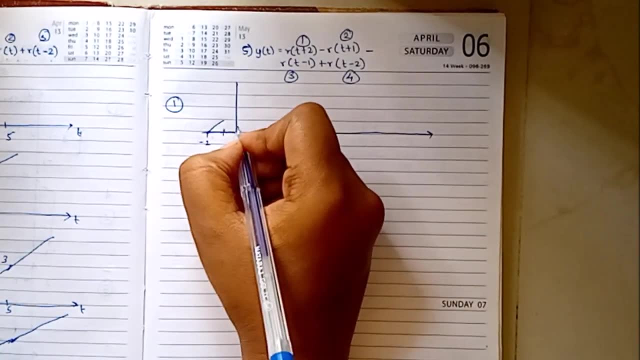 operation row as r of 1, as r of 2 on the left and r of 2 on the right. this is an advanced version of the unit step, so it will begin at minus 2. so at minus 2 the amplitude will be 0, at minus 1 the amplitude will be 1, and so on. 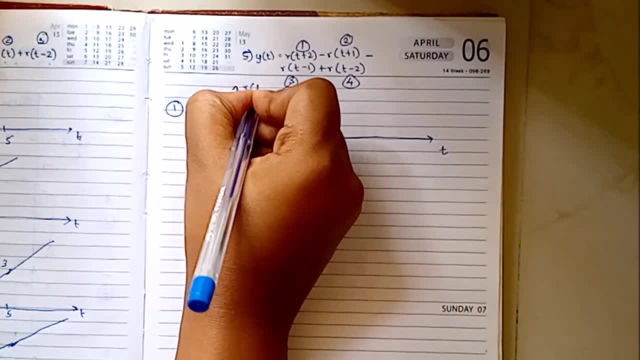 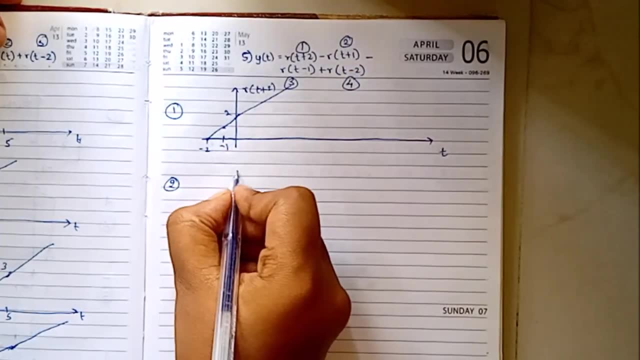 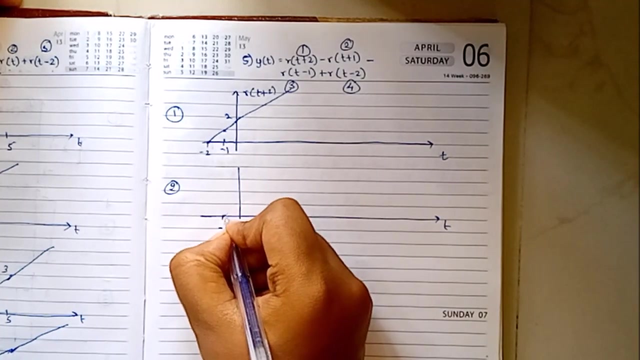 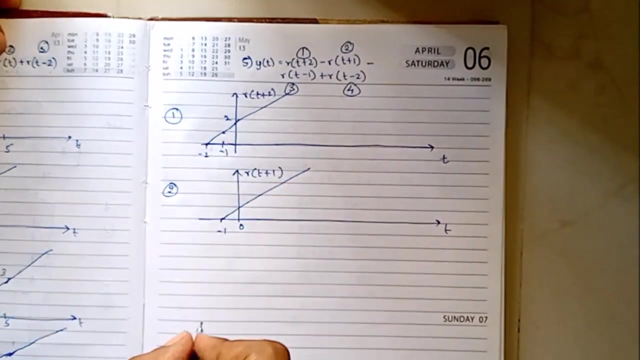 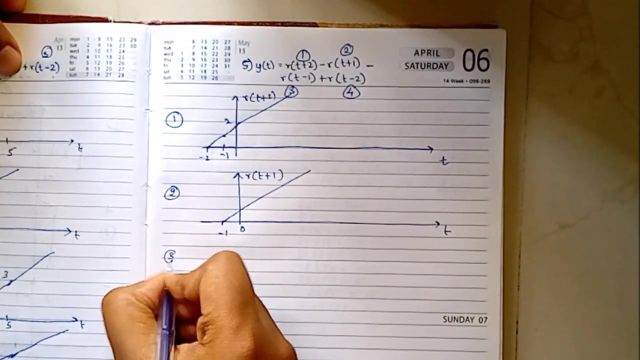 here r of t plus 2. now the second signal r of t plus 1, so it's the advanced version by 1, so it will begin at minus 1. now the third signal, r of t minus 1, which is the delayed version by 1, so it will begin at 1. 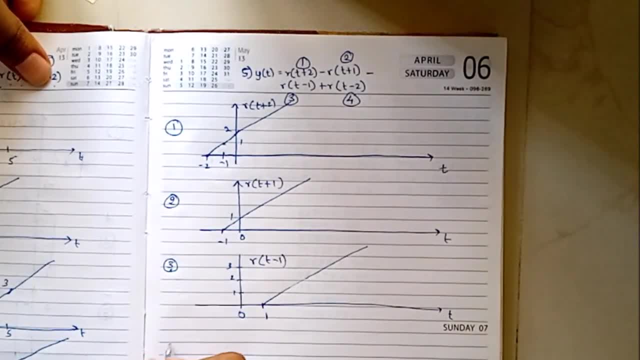 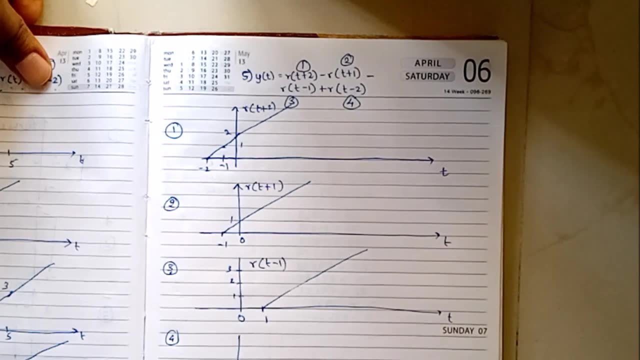 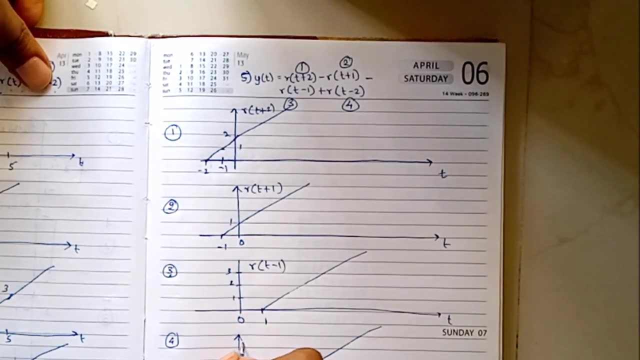 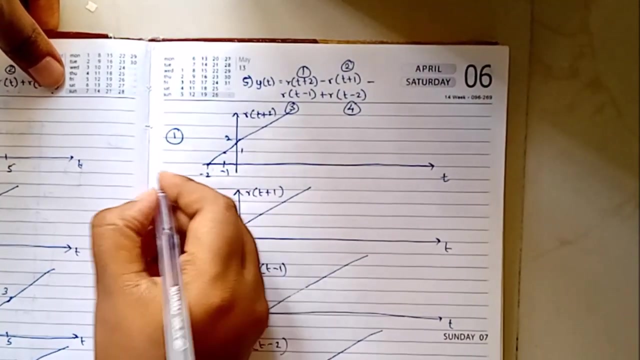 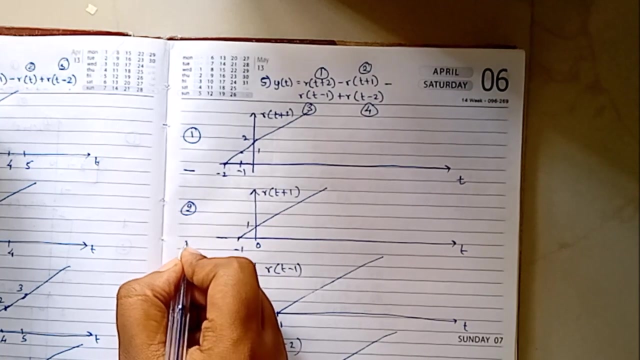 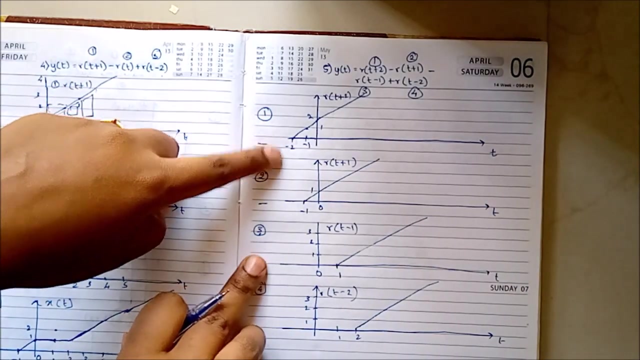 this is r of t minus 1, and the fourth signal is r of t minus 2. so this is r of t minus 1 and the fourth signal is r of t minus 2, so it will begin at 2. so this is 1 minus 2 and 2 minus 3, and then 3 plus 4. so let's start from minus 2, because that's the first one. 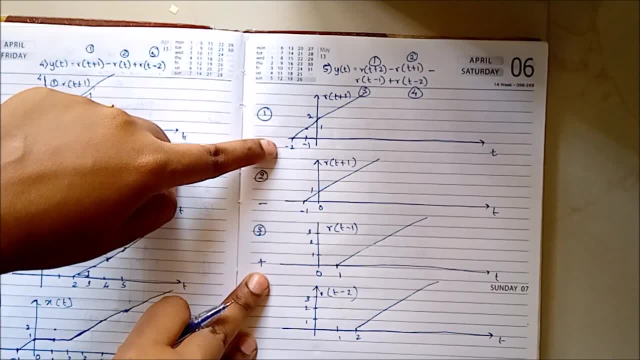 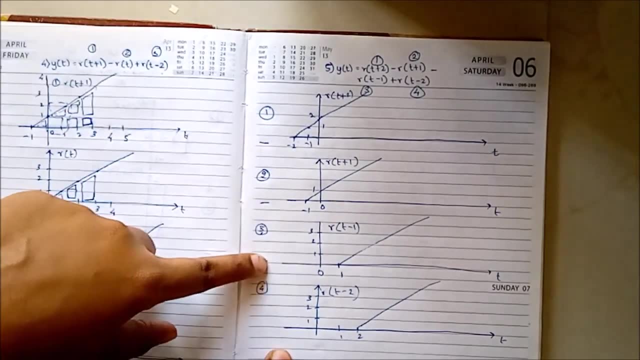 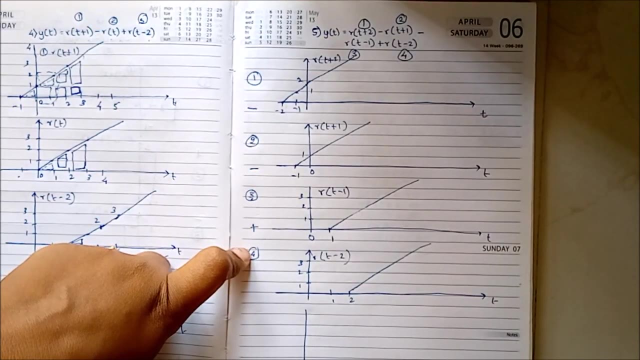 It isаша at minus 2. the first signal amplitude is 0 and the first signal amplitude is 0, so any operation is not going to change. so in a resultant signal amplitude I am going to be 0 itself. it is here at minus 1. 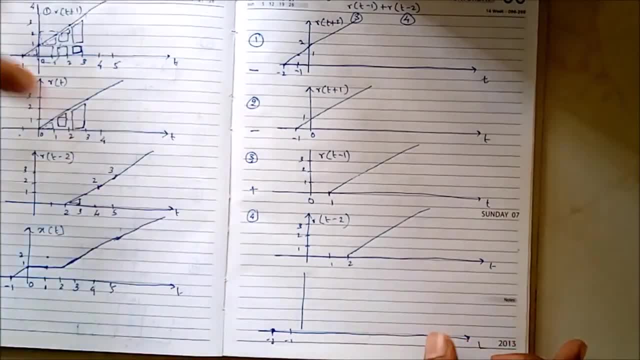 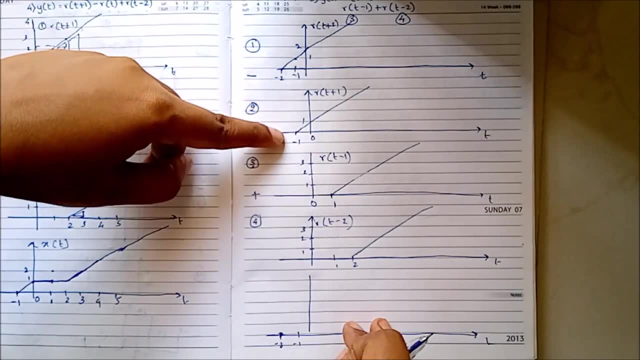 do it carefully: r of t plus 1. also curious, this is r of t minus 1, Preferably principal one, t minus 2 times at all. right now, actually r of t minus 1, and the first point number is 1: one. the first signal amplitude is one. second is zero, third, fourth, all three are zeroes. 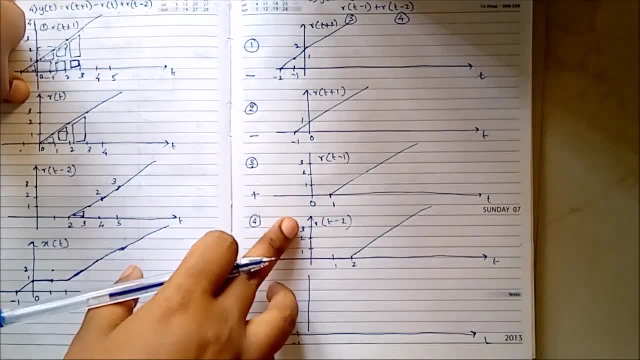 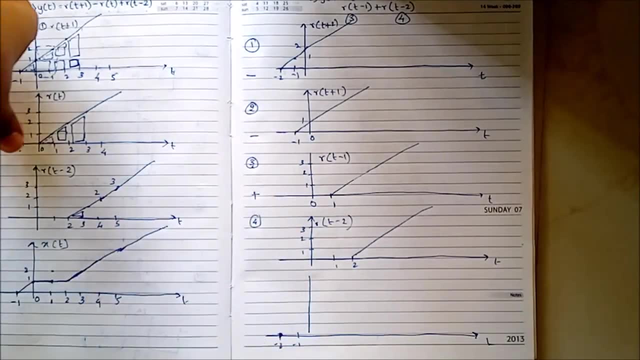 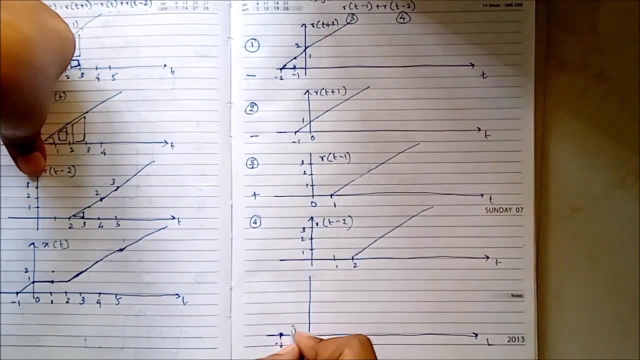 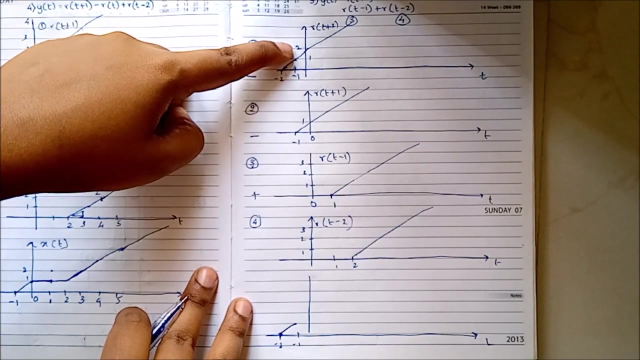 So one minus zero plus zero, and plus one minus zero, minus zero plus zero. so it is going to be one and it's not getting subtracted anywhere this part, so it's going to remain a RAM At zero. the first signal's amplitude is two, second signal's amplitude is one and the rest 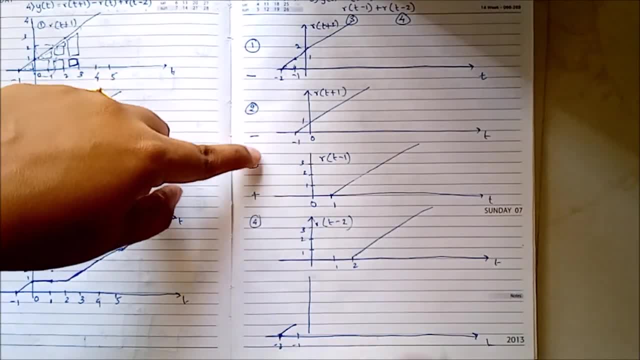 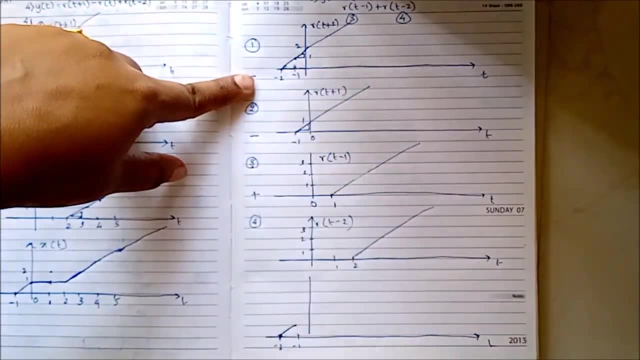 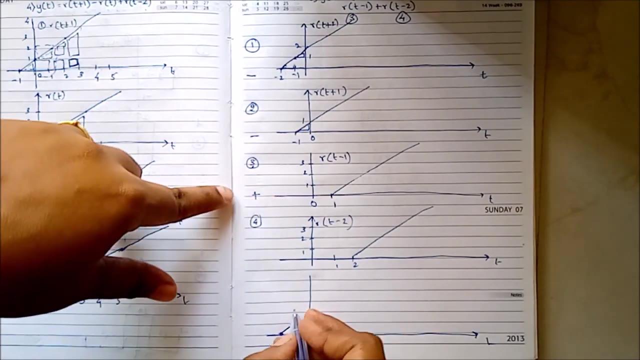 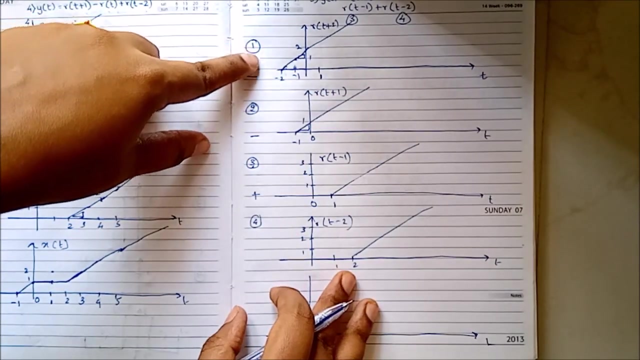 are zeroes. so two minus one is one. and here we can see that this triangular part is getting cut off from the first part. so it is going to be a step. So here the amplitude is one. Now for the point two. At t equal to one, the first signal's amplitude is three. the second signal's amplitude is: 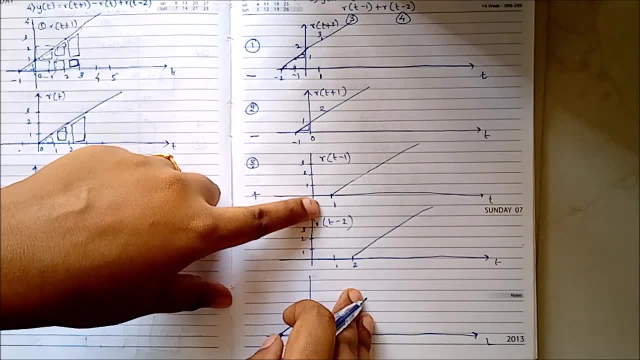 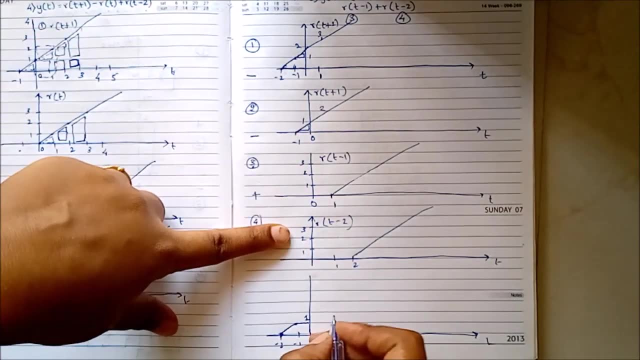 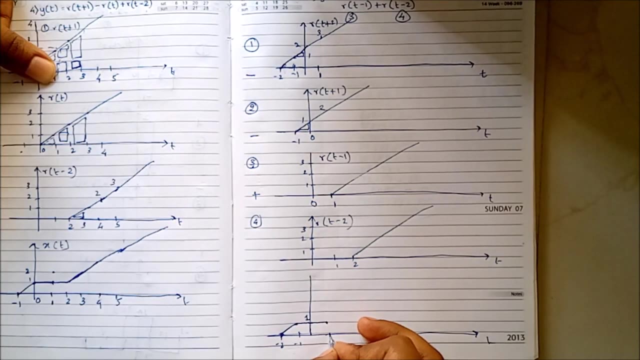 two. the third signal's amplitude is zero and the fourth also is zero. So three minus two is one and the rest are zeroes. so it's going to remain one. So this is at t equal to one, At t equal to two. The first signal's amplitude is one. 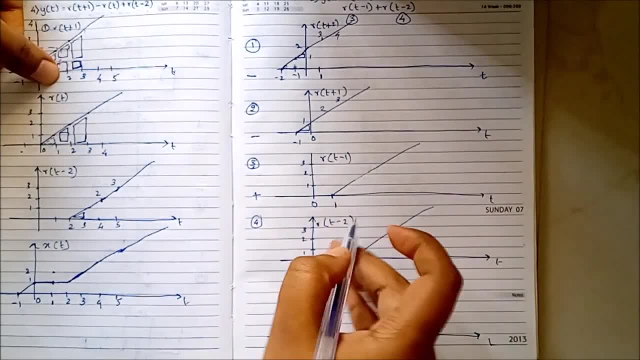 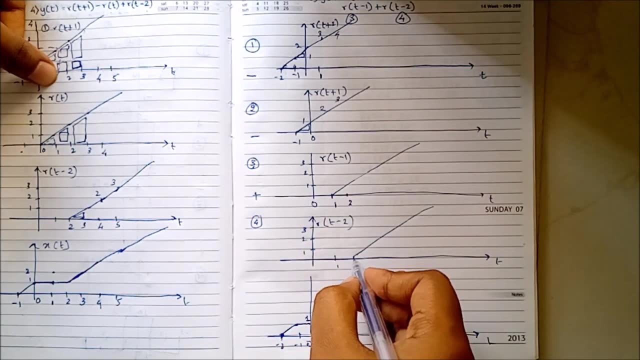 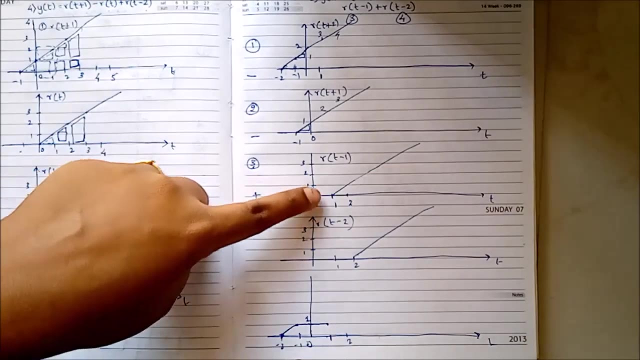 The second signal's amplitude is four. The second signal's amplitude is three. The third signal's amplitude is one. The fourth signal's amplitude is zero. So four minus three is one, one minus one is zero, and zero plus zero is zero. 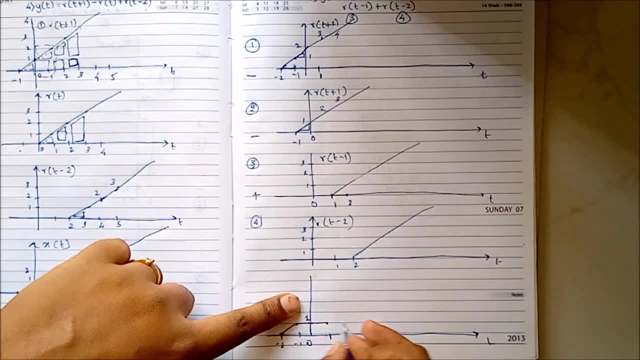 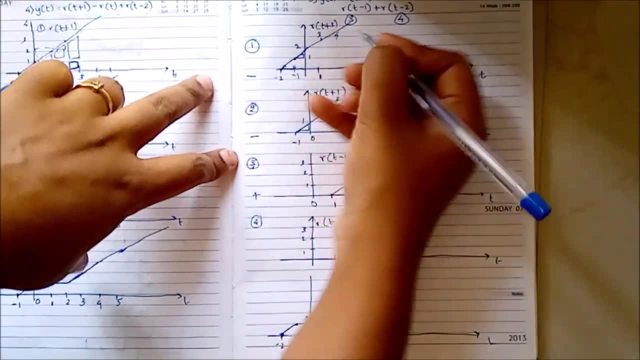 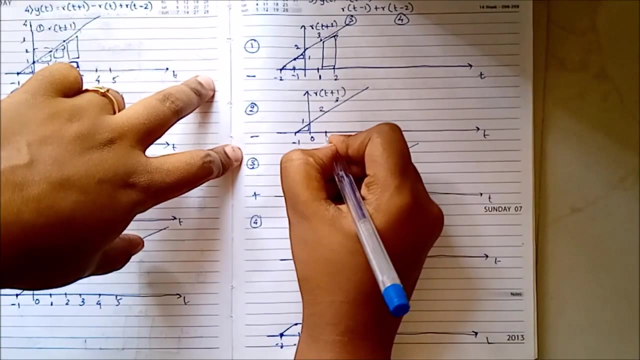 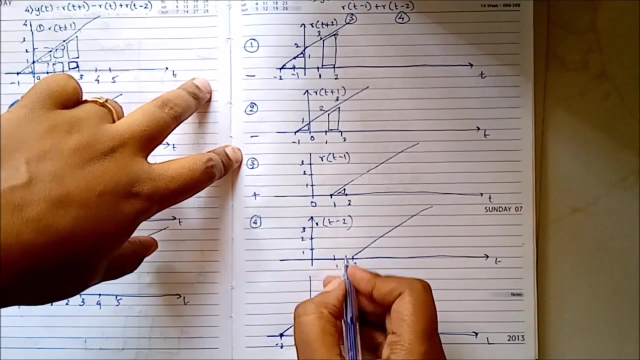 So at two we can see that the signal is going back to zero. Here we can see that this is a triangular section. till two and here at two this is again the same shape. Here at two it is a triangular shape and here at two it is a zero shape. 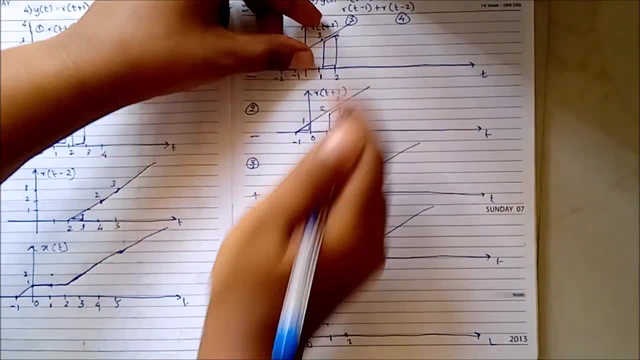 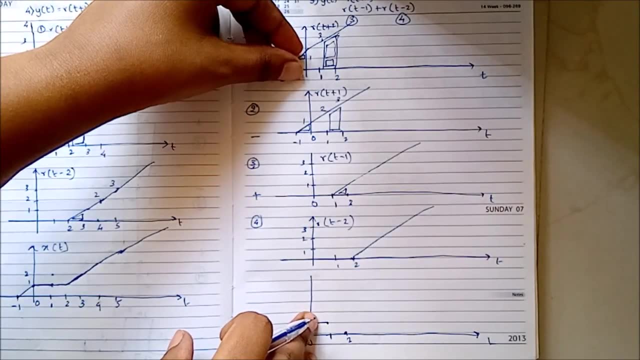 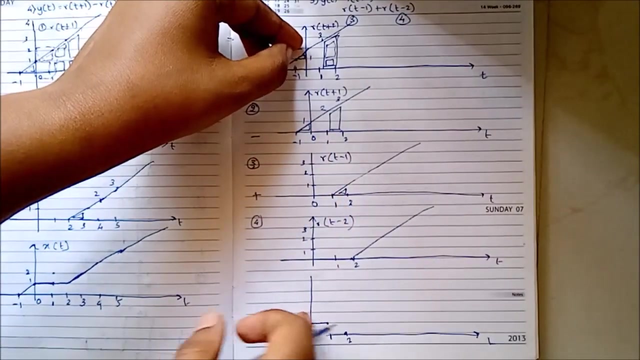 So here we can see, this part of the signal is getting subtracted from here, So only a step signal is getting subtracted from the second. step signal will remain, and this we are again subtracting from this, we are subtracting this triangular section. so because of that, we are getting a zero and this shape will get inverted. 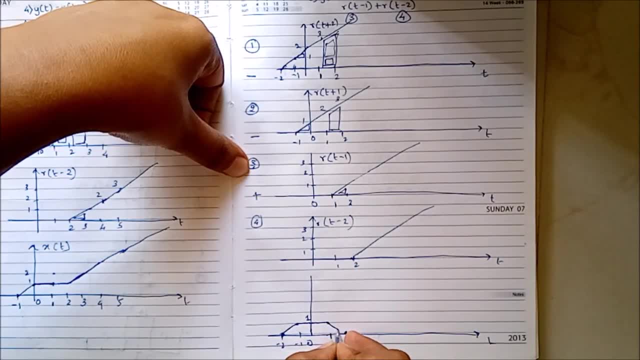 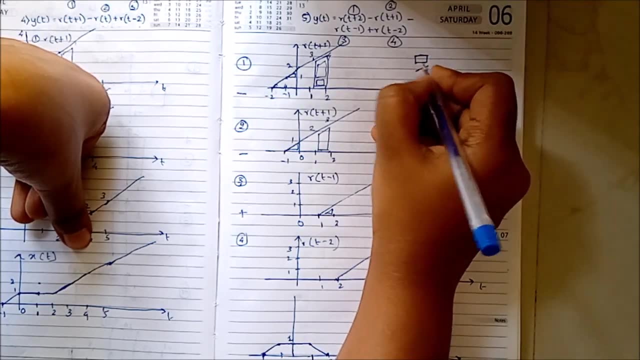 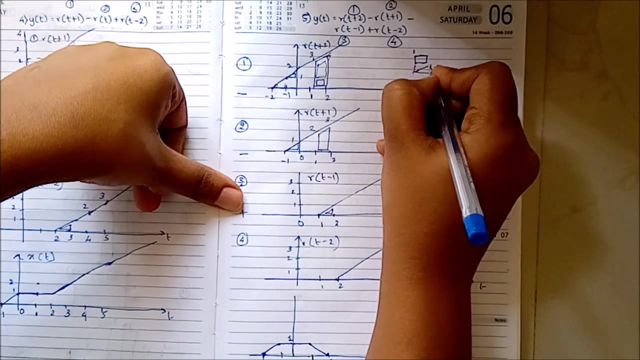 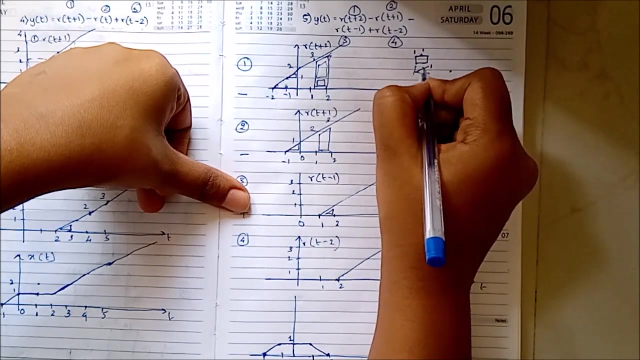 because if we subtract a ramp from this step, so it will be suppose we consider this amplitude as 1 and here this amplitude as 1, so 1 minus 0 is 0, and if we consider this intermediate point as 1 and here as 0.5. so here we will just draw the resultant. 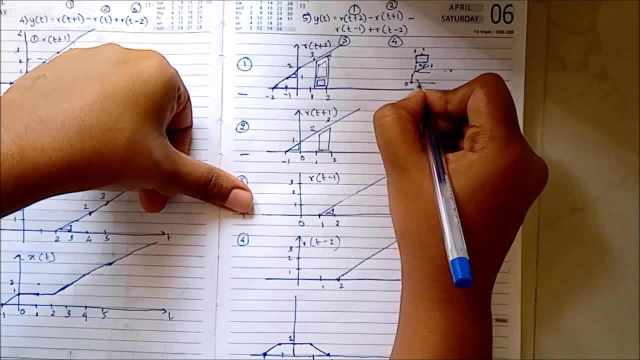 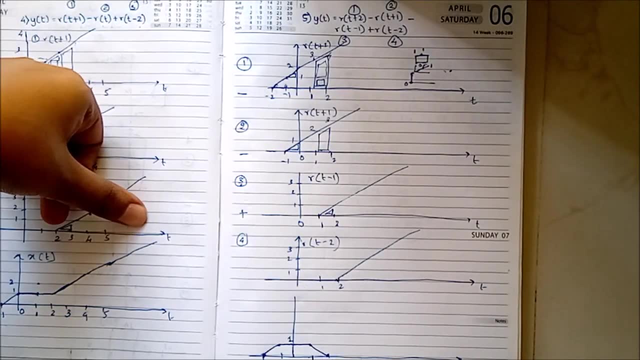 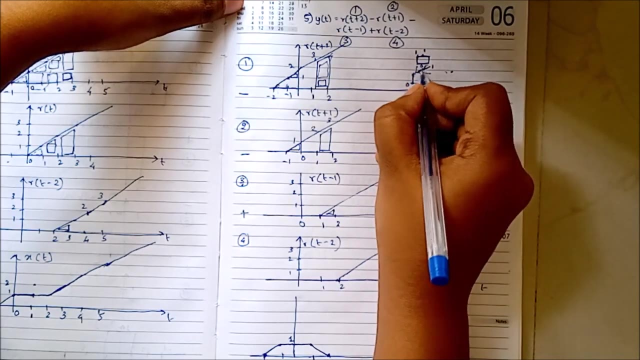 so here we will just draw the resultant. so this is 0. so 1 minus 0.5 is if we consider this as the rectangular signal or the unit step, and if we consider this as the unit ramp and we try to subtract the second one from the first one, so it will be at 0. 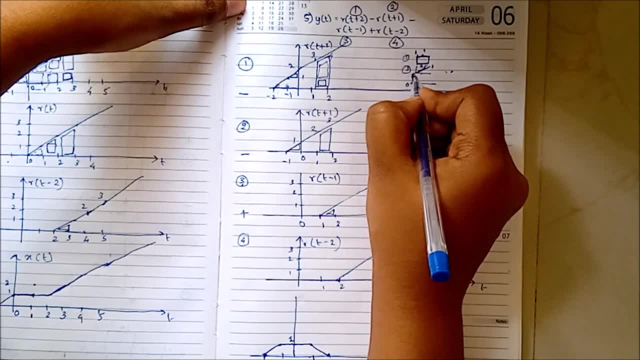 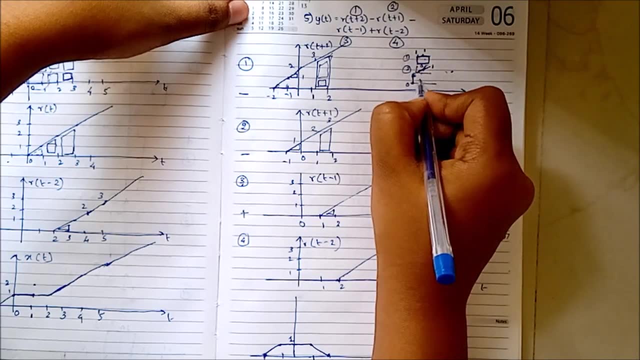 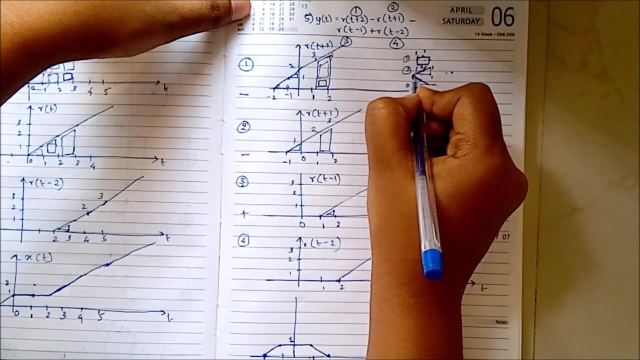 suppose 1 minus 0 will be 1, 1 minus 0.5, which is the intermediate point between 0 and 1, will be 0.5, and 1 minus 1, that is, at 1, the point will be 0. so it will be an inverted ramp. so the shape will be. 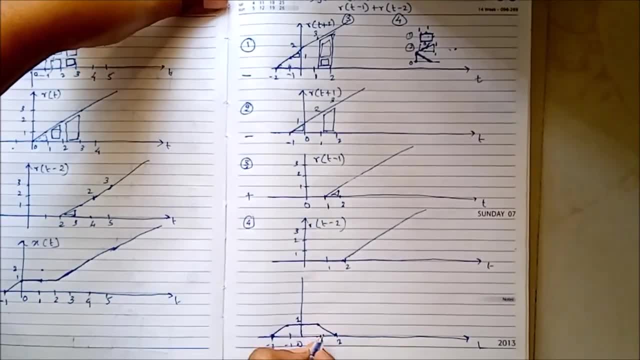 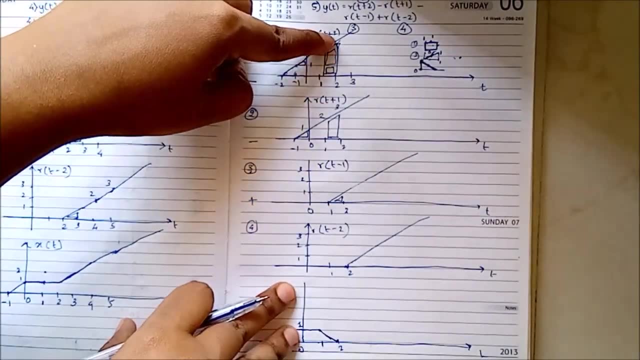 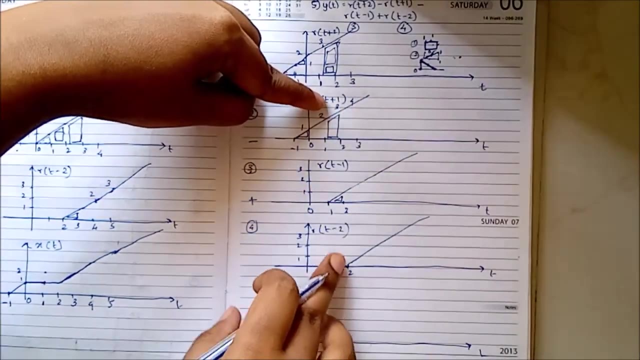 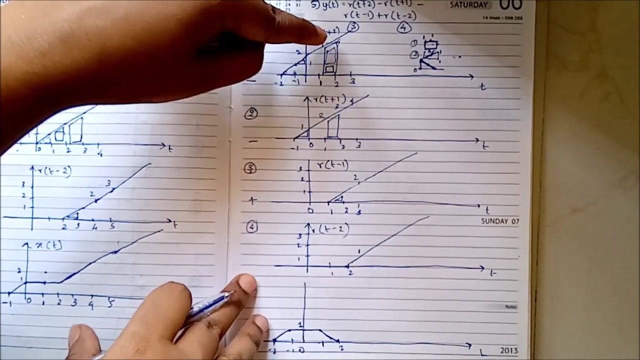 just the opposite. so we get this kind of a shape: the resultant signal, your 3nd signal, the first signals amplitude is 5, the second signals amplitude is 4 and this next by choosing: And the third signal's amplitude is 2 and the fourth signal's amplitude is 1.. 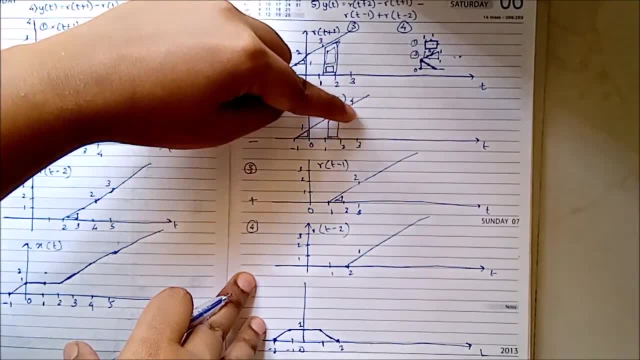 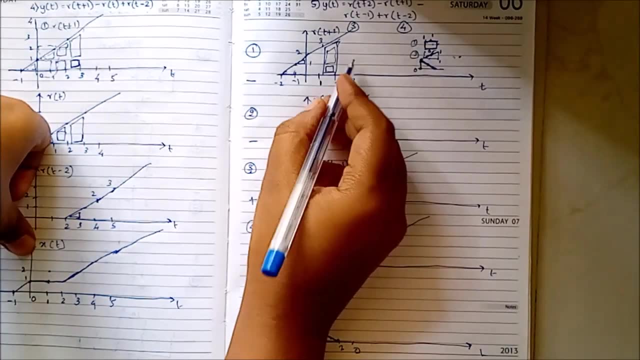 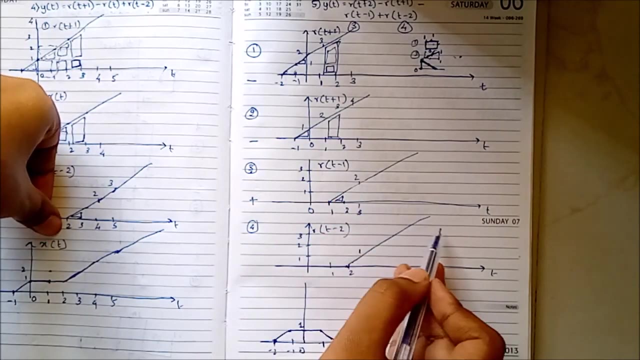 So 5 minus 4 is 1, 1 minus 2 is minus 1, minus 1 plus 1 is 0. So this point is going to be 0 and this is going to continue for all the other points, because the shape is going to continue. there is no 0 point in the middle. 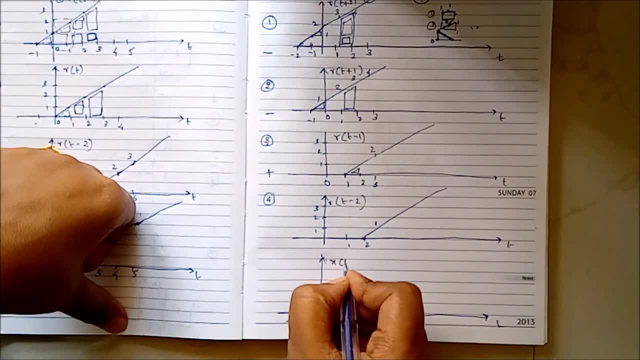 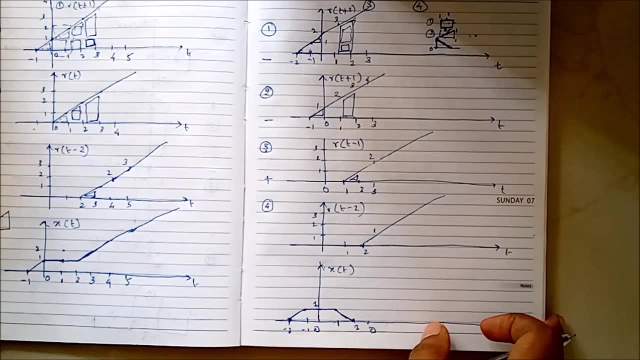 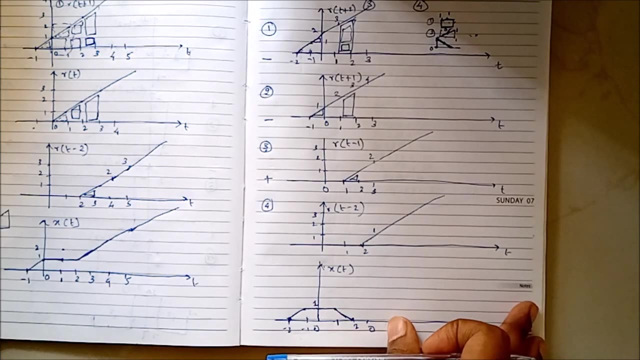 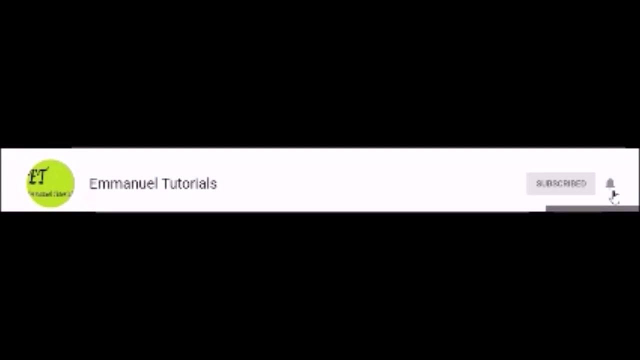 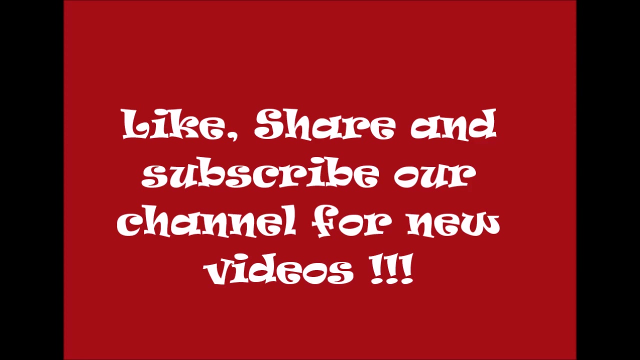 So this is the resultant signal which we require, which is x of t. Thank you for watching the video. If you have any doubts or comments, you may mention it. Do like, share and subscribe our channel for more videos. Thank you you.